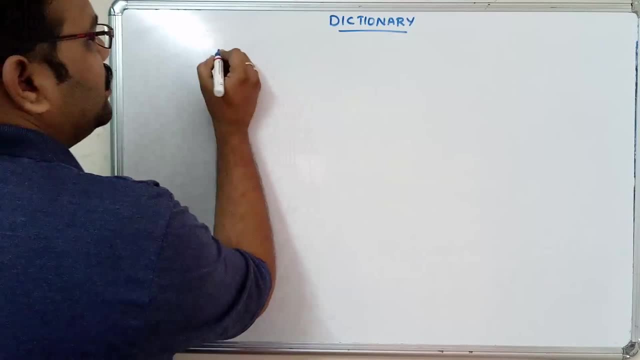 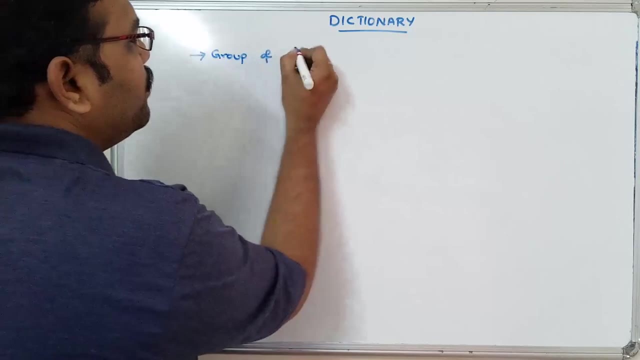 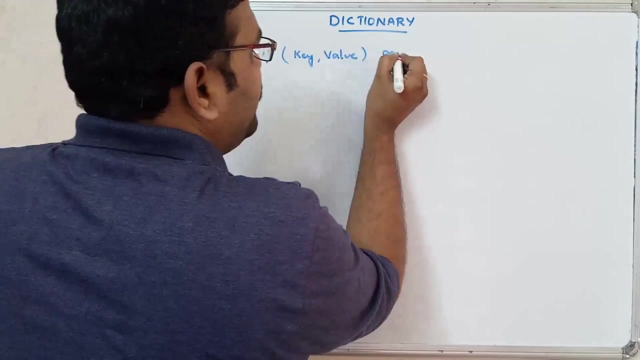 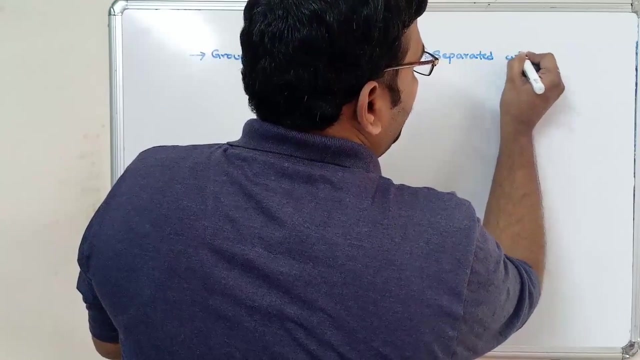 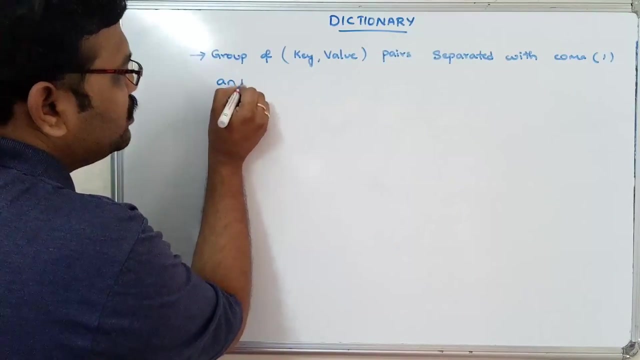 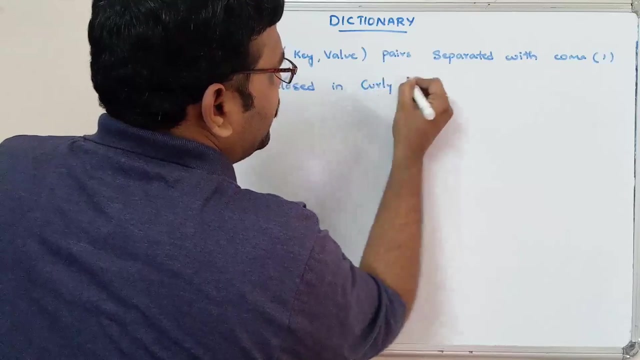 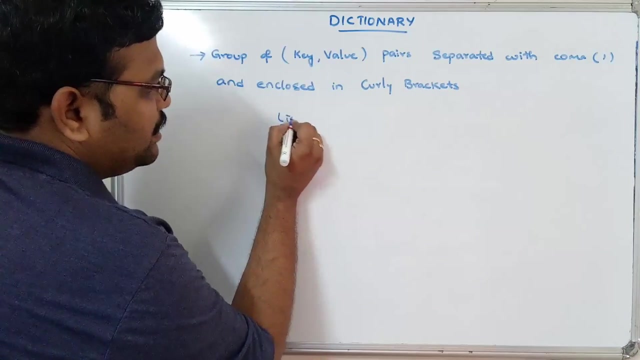 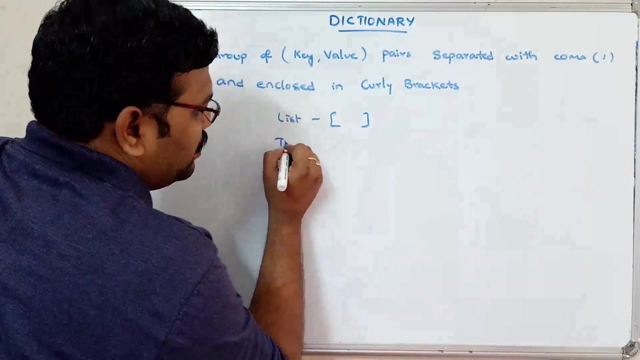 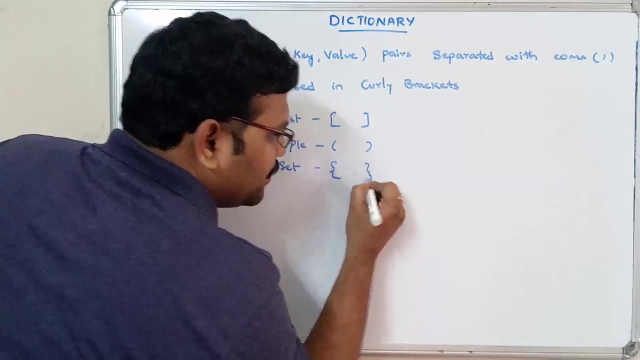 group of key value pair separated with comma and enclosed in curly braces. right, this is important- curly braces. so, whereas list will enclose the multiple elements which are separated with the comma in square braces, and tuple will use the parentheses. in a set, then we will use the curly braces and in the dictionary, 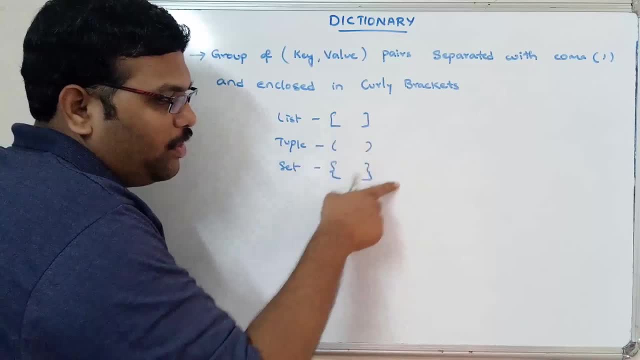 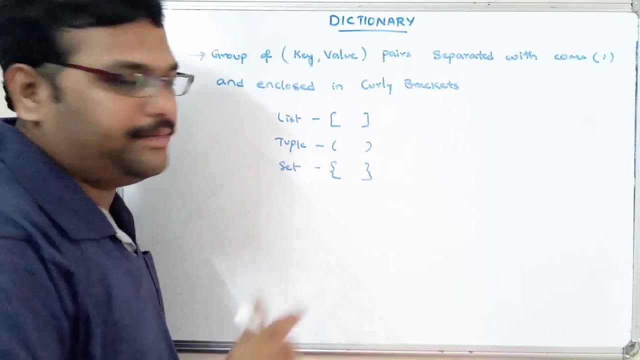 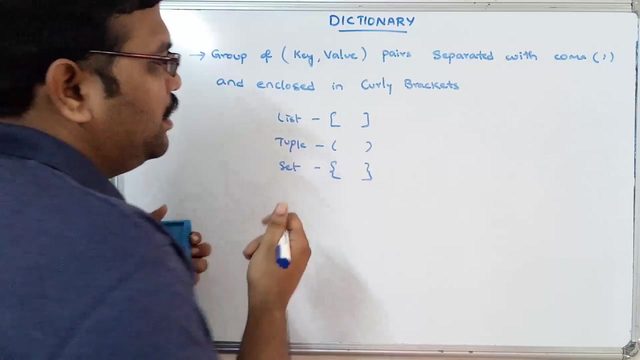 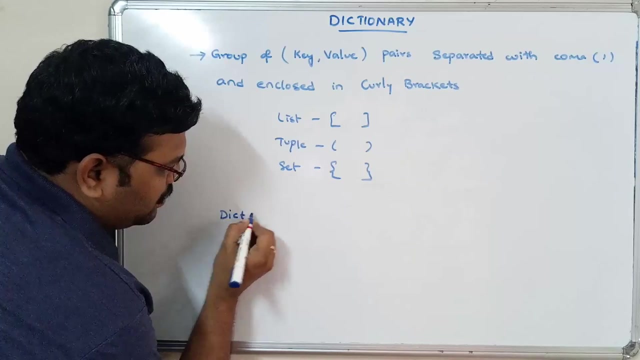 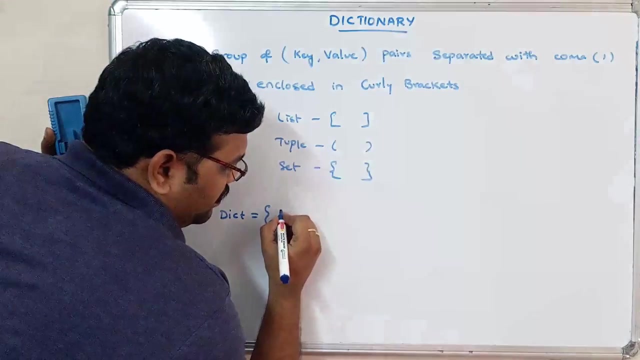 similar to the set. it will also. the elements of a dictionary will also be enclosed in curly braces, but in terms of key value pair. key value pair, right? so this is the definition, simple definition we can say about this dictionary: right, so let us create dictionary is equal to curly braces. so here we have to. 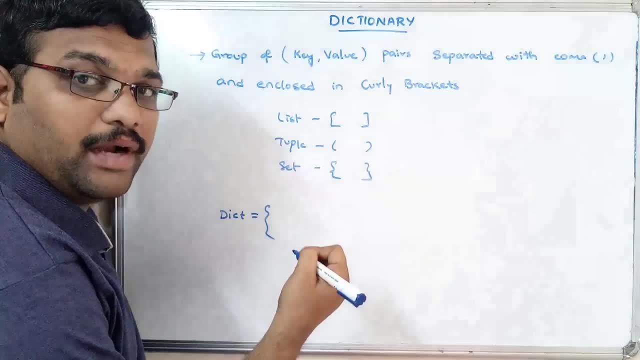 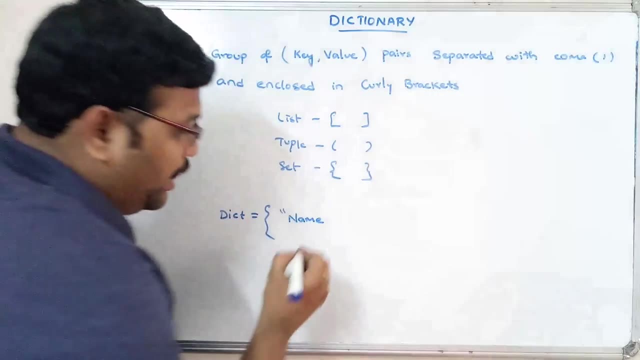 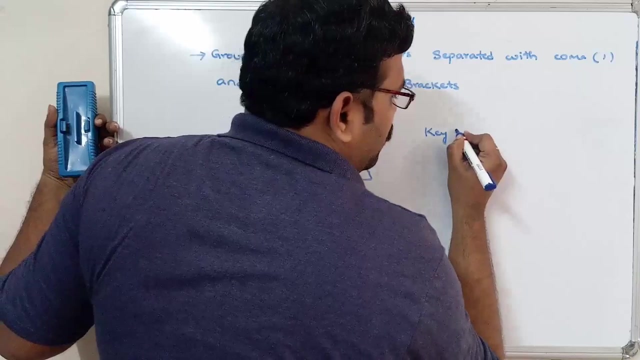 give a key followed by the value right. so let us take an example: name. name is a key and these key values are the key values of the dictionary right. so let us take one. our key of the dictionary right here is the dictionary Coach found that if your entire correspondence is shared with the background TEAM 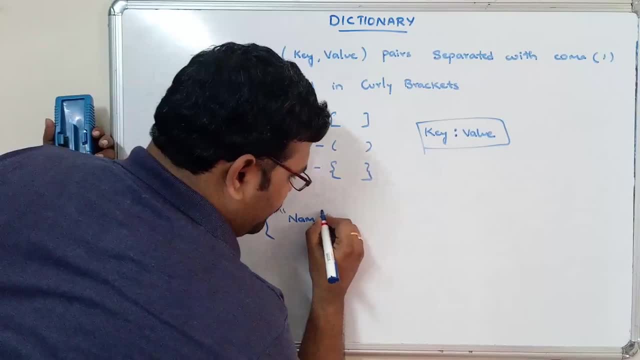 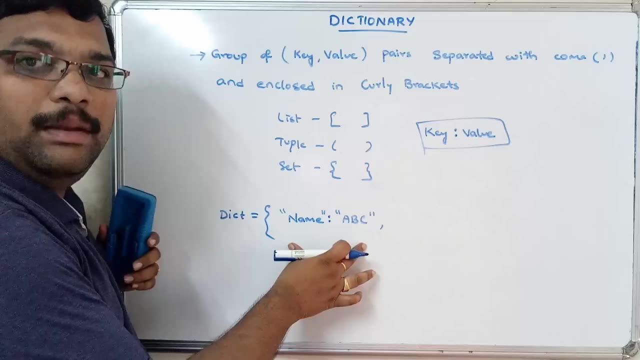 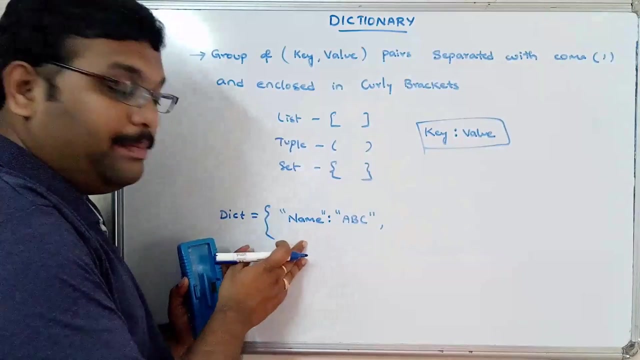 bench. it will be viene, Esteban, you to give an example, right, so it is workflows. okay. for example, if you and your calendar have got a document which is called as aолот, Click on Add on�� and add the code: events right here, moments, whatever. its a browser or something like that. something else can be. 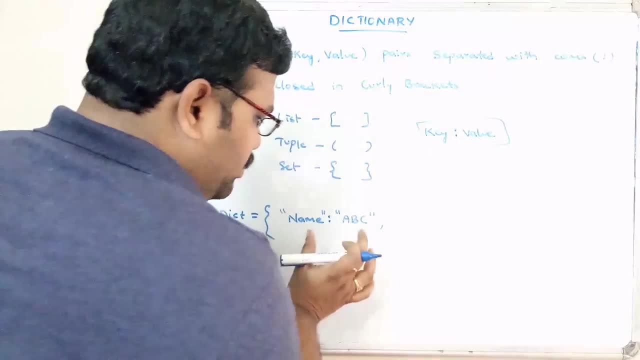 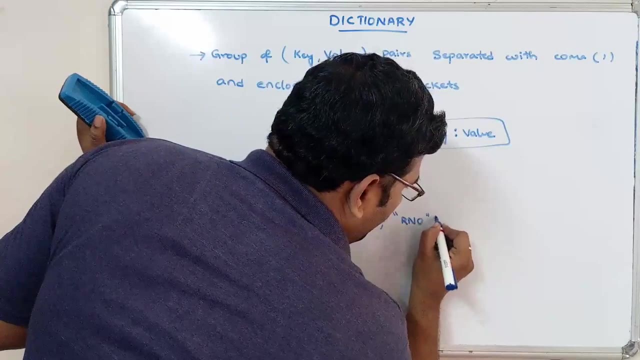 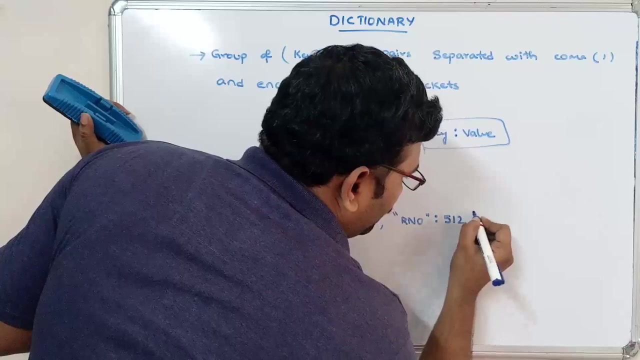 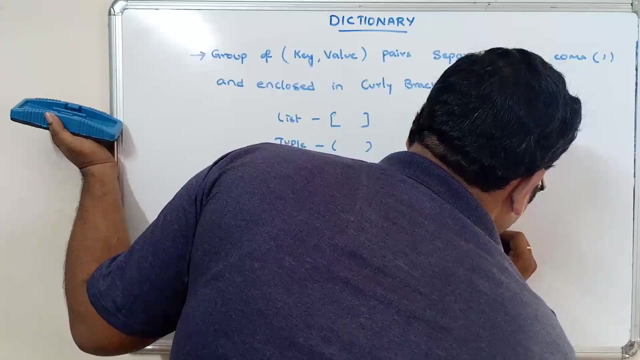 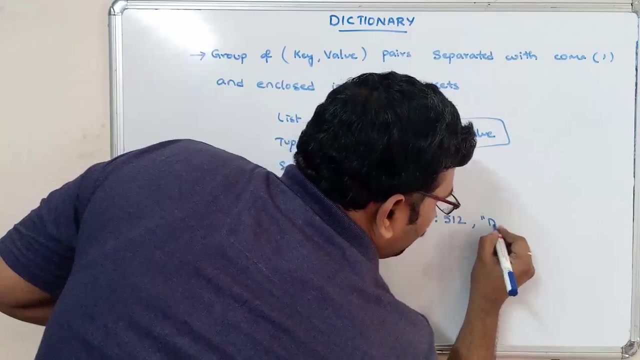 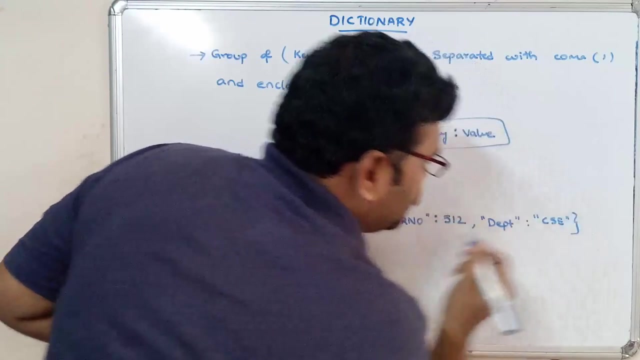 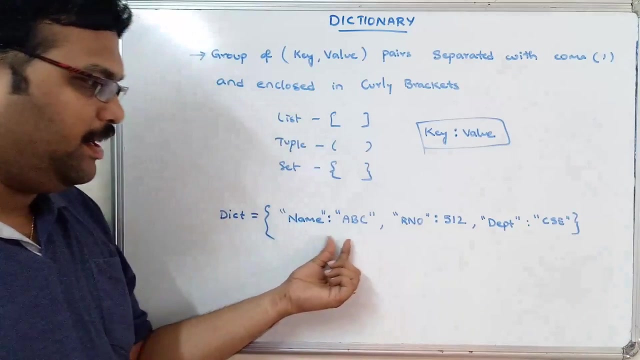 done, and so this we need with this debugging. I just wanted to show you that is treated as a values. so these forms a key value: P R, number, arrow number, comma, department six. so here the dictionary consists of a key value base, separated with a comma, right, separated with a comma and closed in a square. 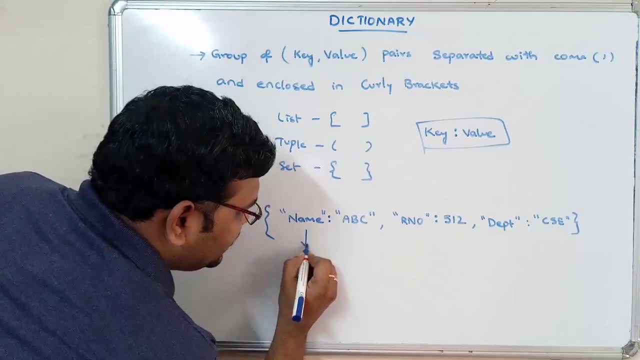 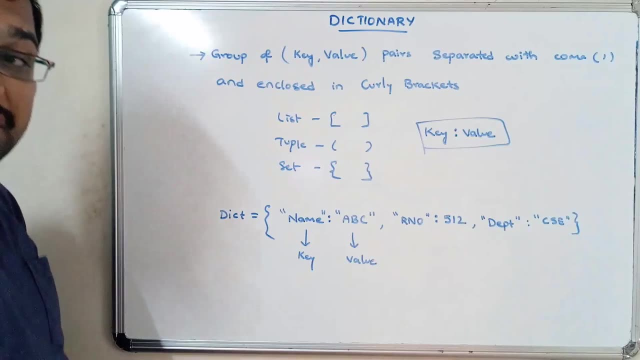 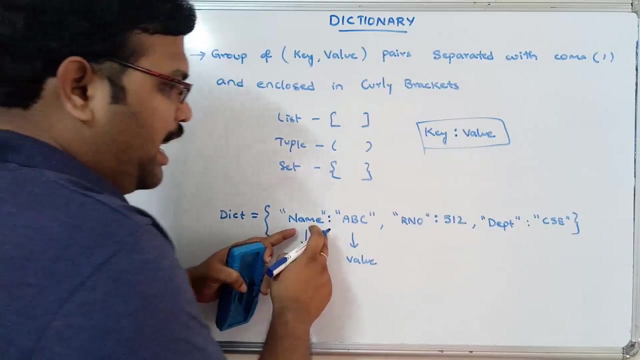 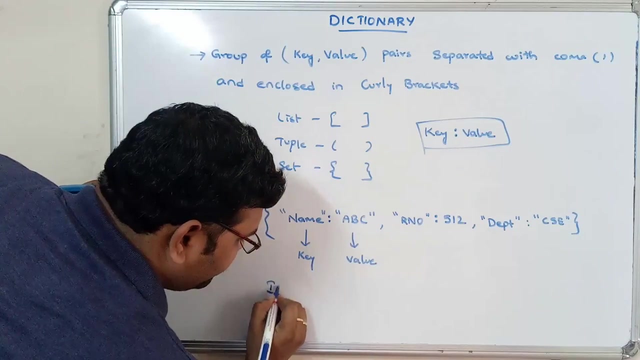 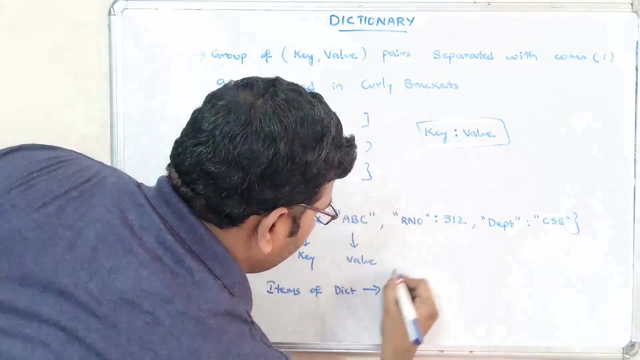 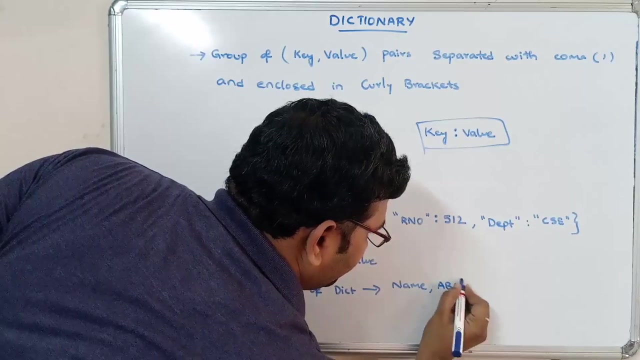 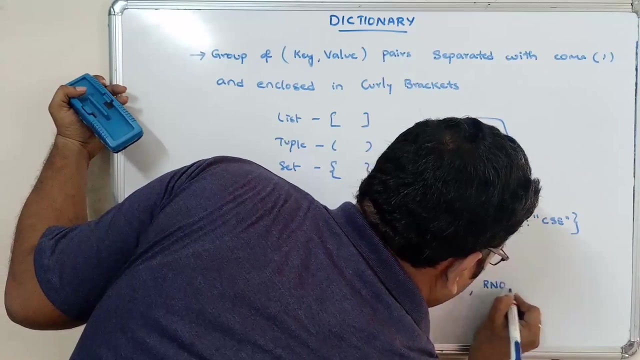 bracket. so this is a key. this is a hope. you understood this one. this is a key, this is a value, right? so we are having three elements, so here we call these as items. items of dictionary are named ABC, so it forms a tuple. ok, comma, R number suppose. 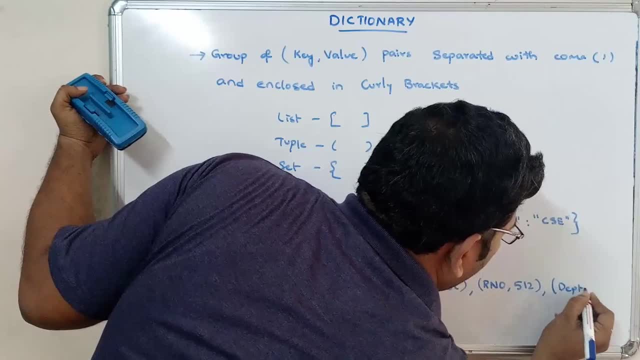 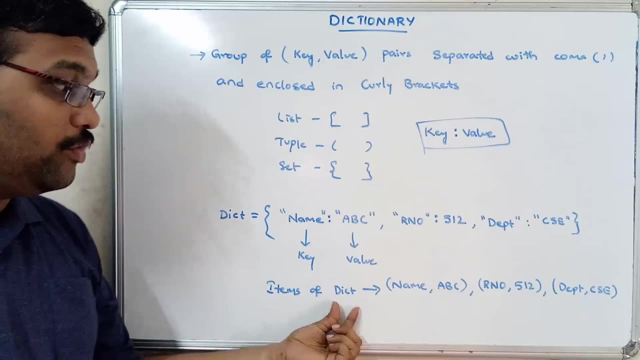 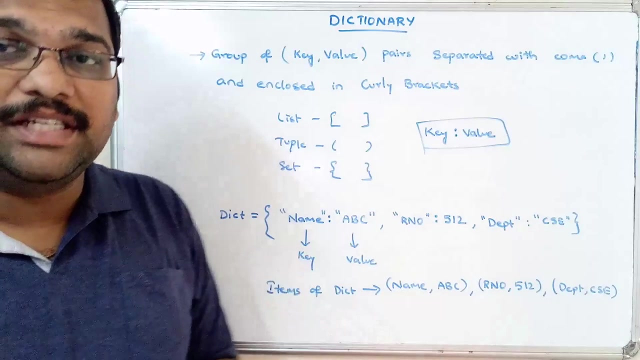 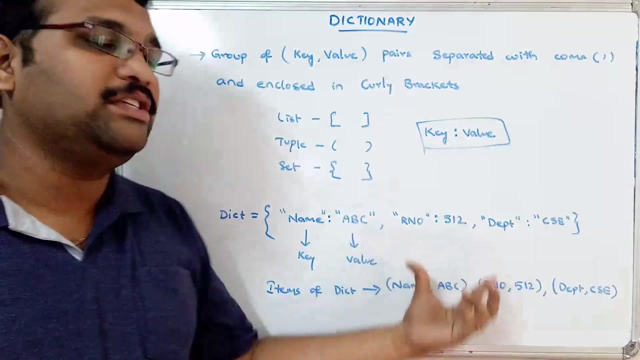 I call. come on bptc e tip right. So these are the items of a dictionary, so we should not call them. Call these as elements. We will call these as items. So why? items means there is a function called items, So there is a method called items which will display all the elements of the dictionary so we can. 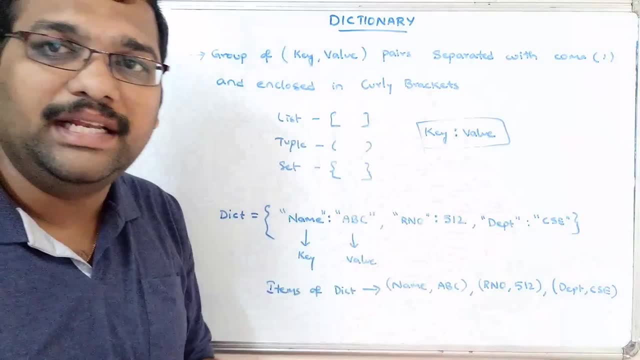 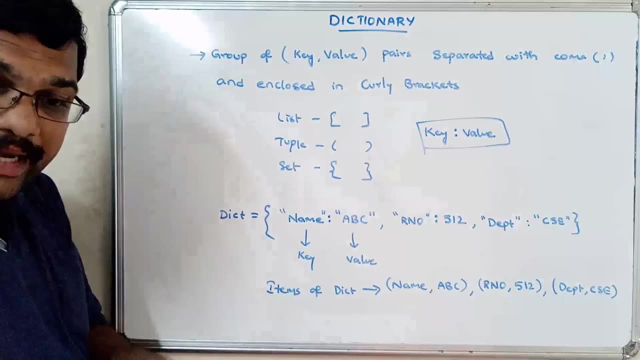 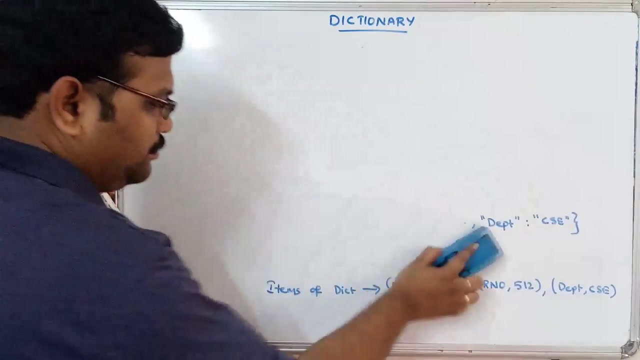 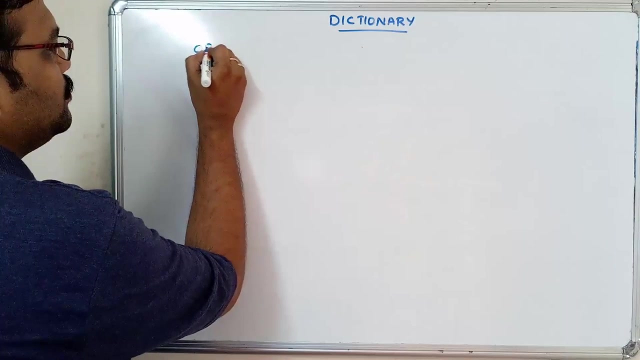 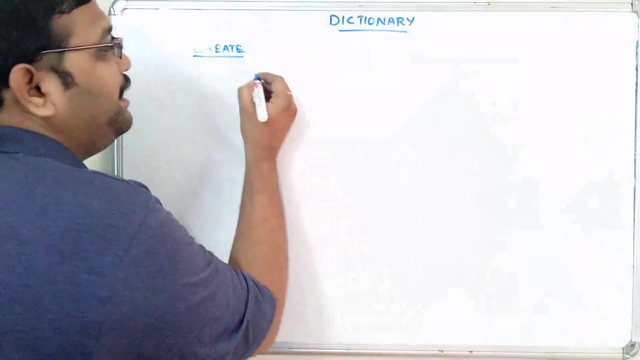 Treat these elements as an item so that we can easily implement that thing. okay now. So how to create a dictionary? Right, so we'll see how to create a dictionary. So how to create a dictionary. so an empty dictionary is created as: so this is an empty dictionary. 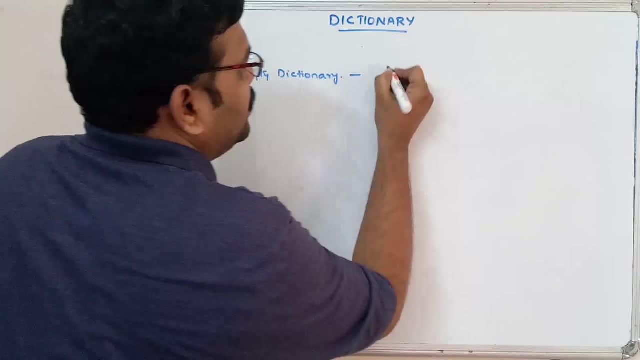 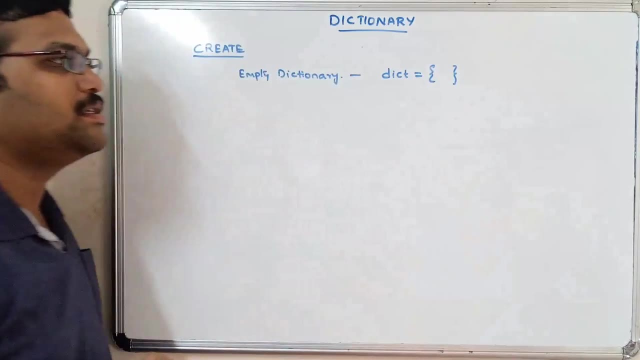 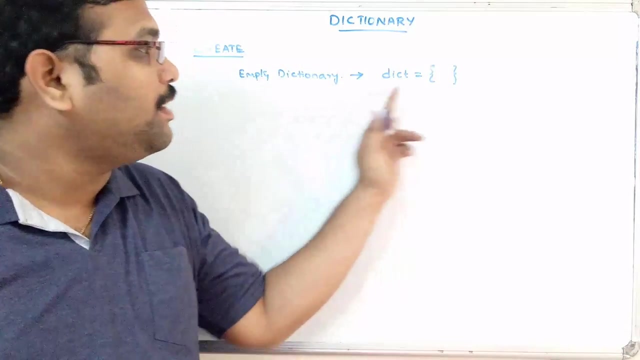 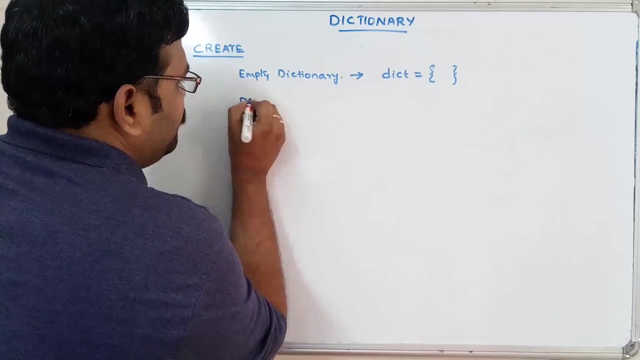 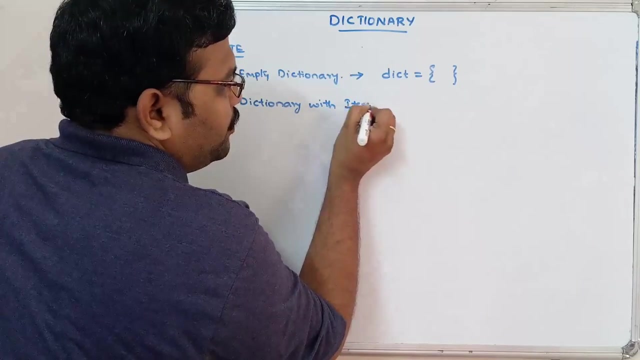 So this is how we can create an empty dictionary. Some DICT is equal to open curly brace closer to this. so this is how We can create an empty dictionary Right now. so how to create a dictionary with elements, Dictionary with items. okay. so for that we have seen. 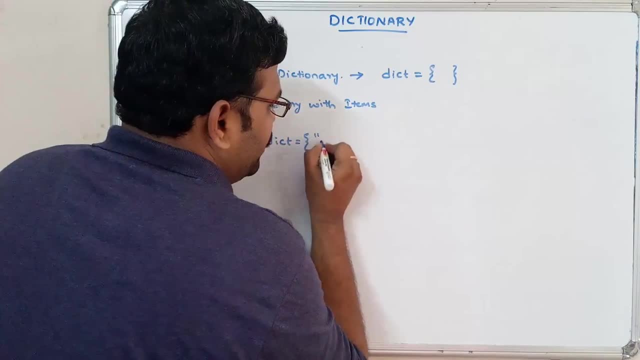 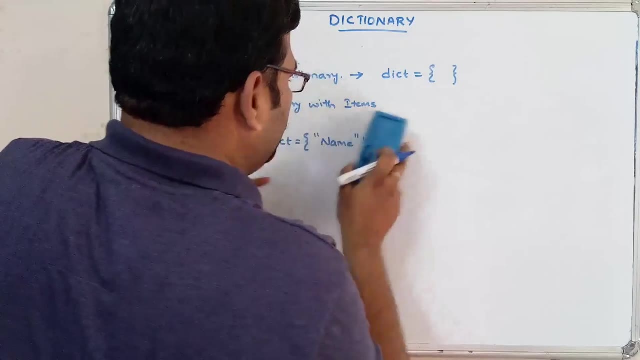 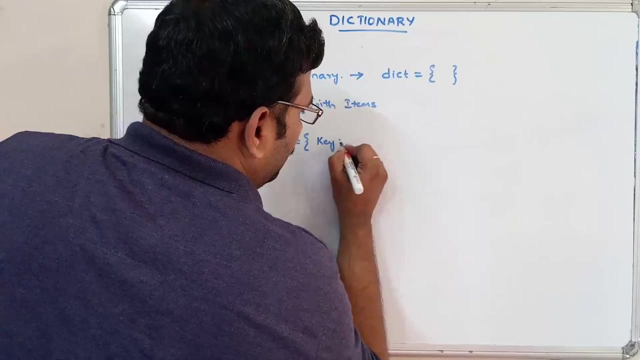 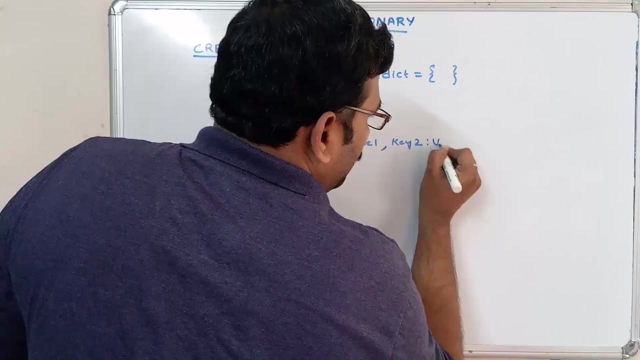 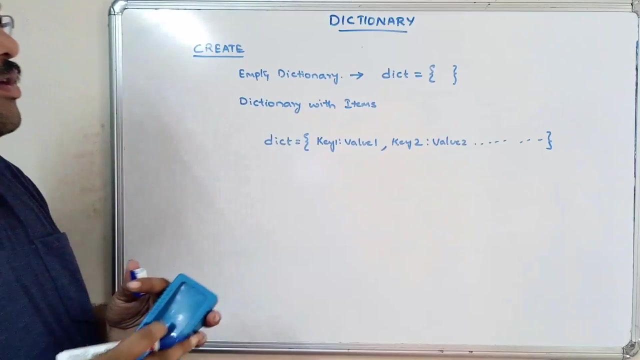 So DICT is equal to open curly brace so we can go with the Key colon value. I will write the syntax here. So key colon value 1, comma. key 2, colon value 2 and so. So this is a syntax for creating a dictionary with the multiple key value pairs and 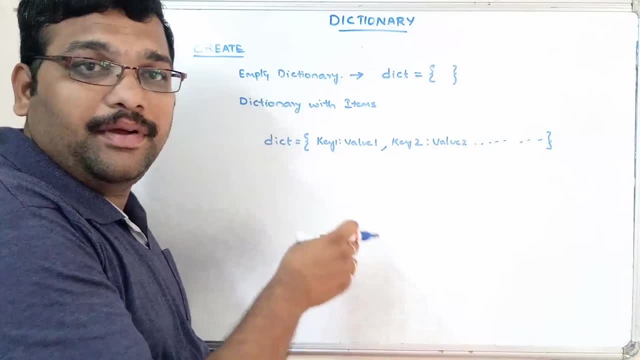 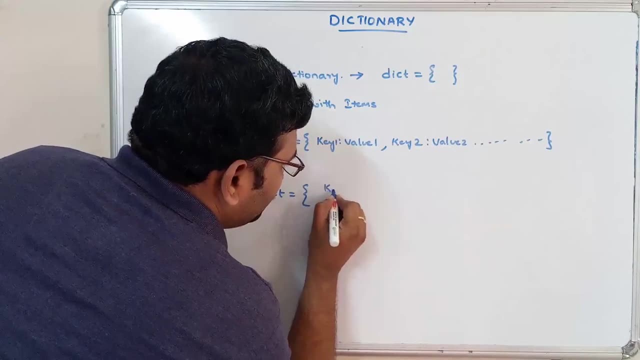 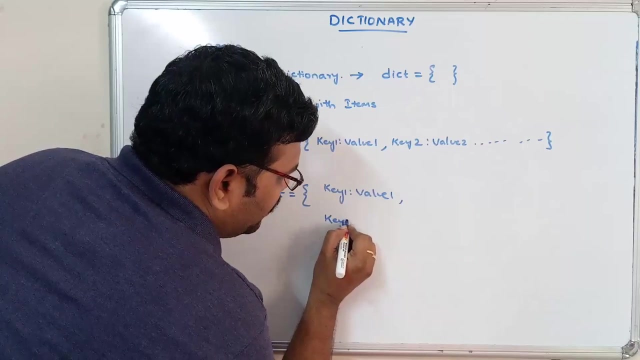 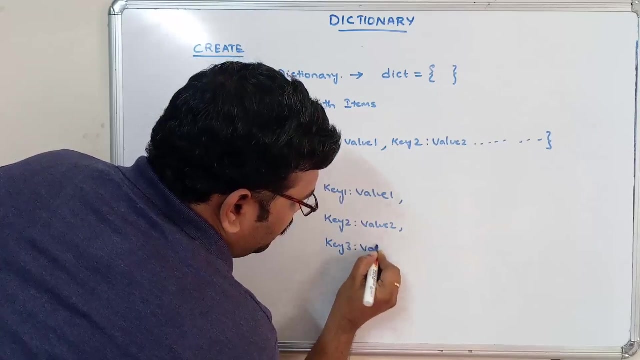 If you want to write it in a single line- I mean multiple lines- we can also write it as DICT is equal to so write the statement key. I mean write all the pairs in its individual lines. Okay. colon value 2. Key 3. colon value 3. 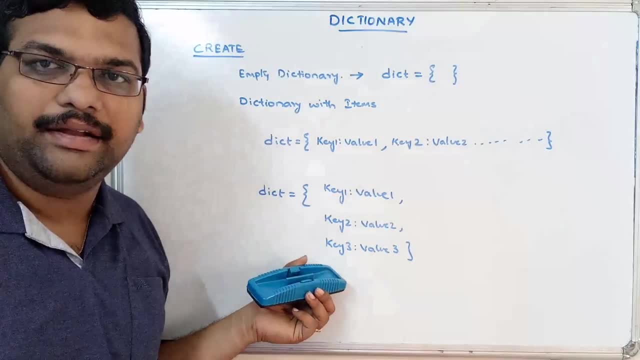 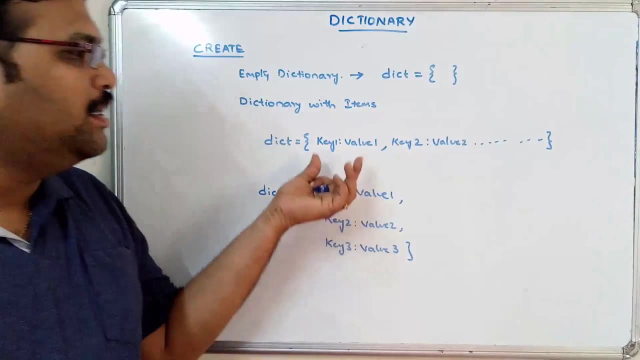 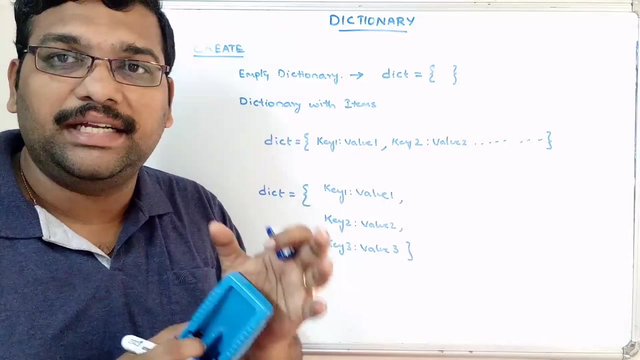 So, in similar way also, we can Create a dictionary. so writing the key value pair in single line, every key value pair in a single line, Right, so this key value can be any data type. If it is a string, we have to enclose that string in between the single line. 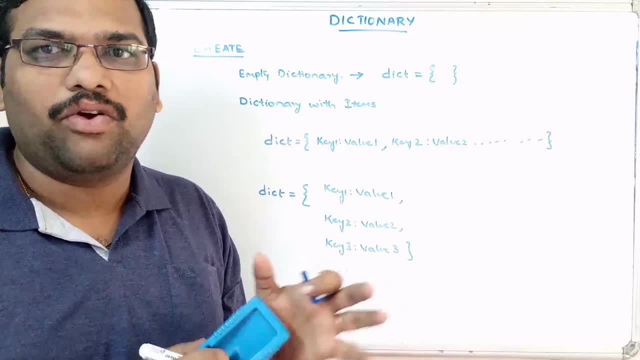 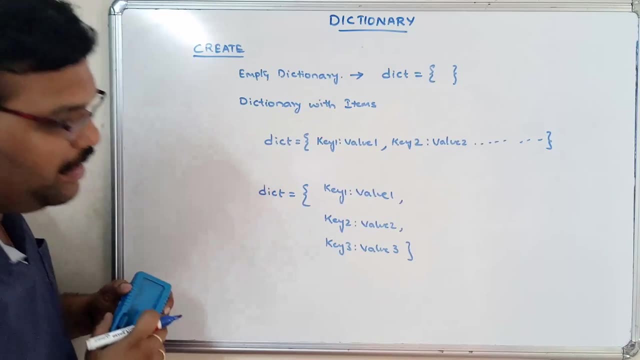 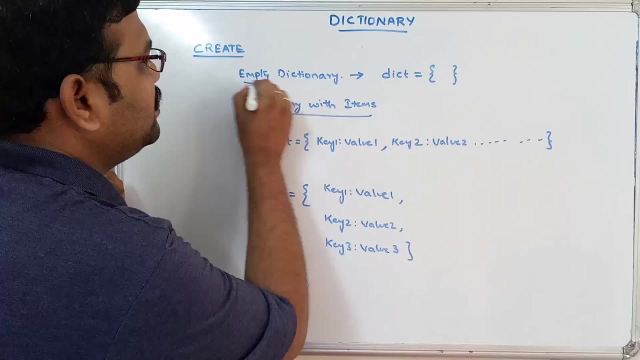 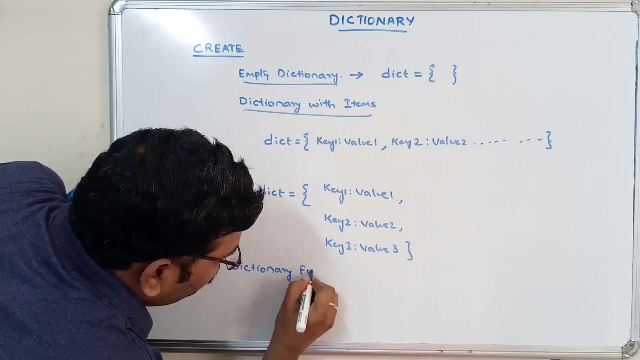 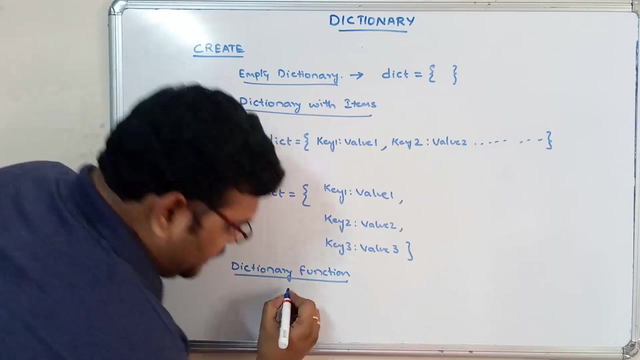 The single quotes or a double quotes. So that's a common procedure. So, and this is how we can create a dictionary, and also we can create a dictionary by using the dictionary function. So this is items. this is an empty dictionary. next, Dictionary function. So there is a function called DICT. 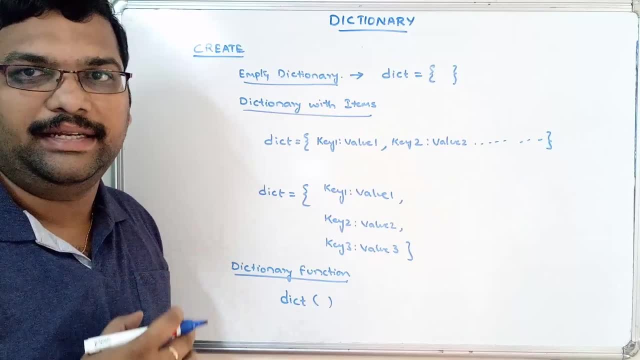 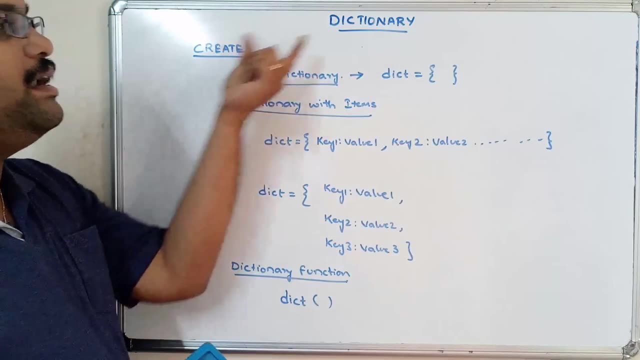 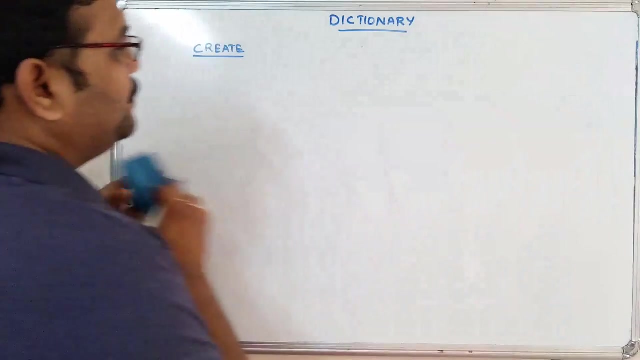 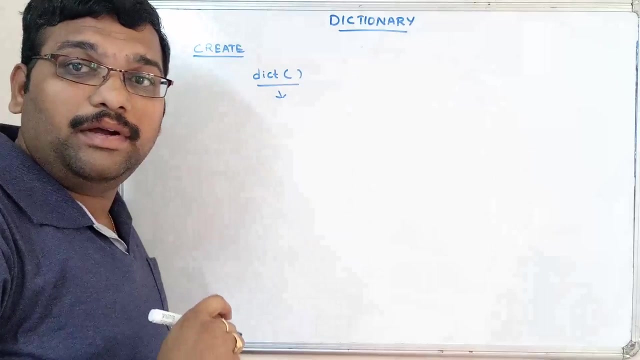 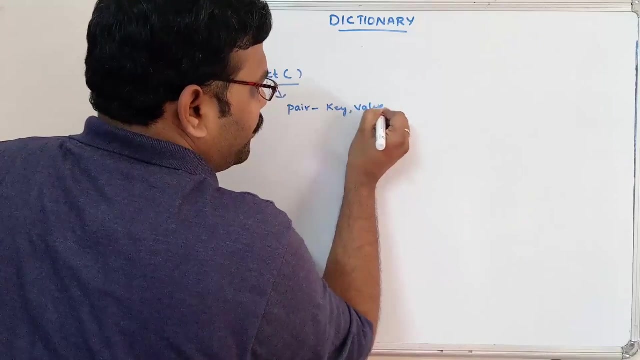 Which is used to convert into the dictionary. it forms a key value pairs, So we can use this dictionary function to create a dictionary. So we will see how it will be created. Dictionary function- Dictionary function. so here we have to give a pair of Key values In tuple. 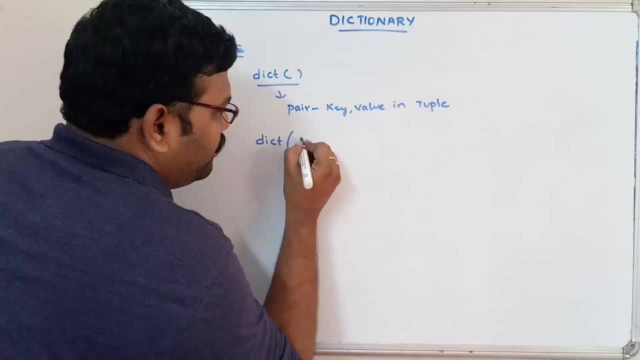 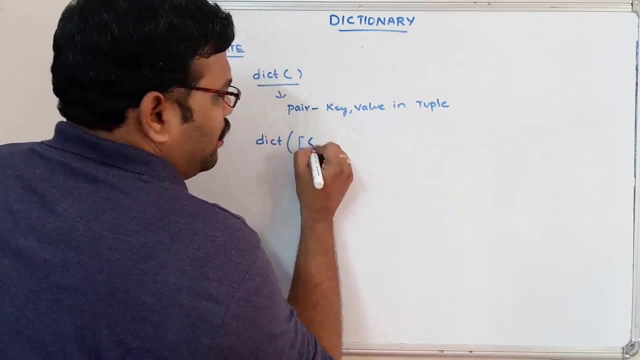 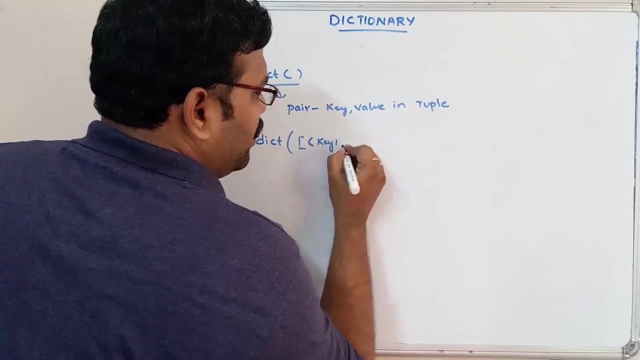 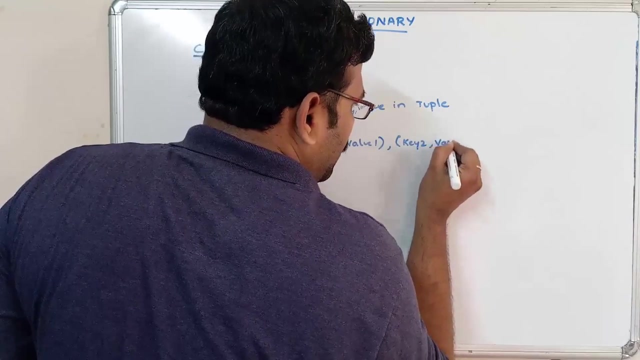 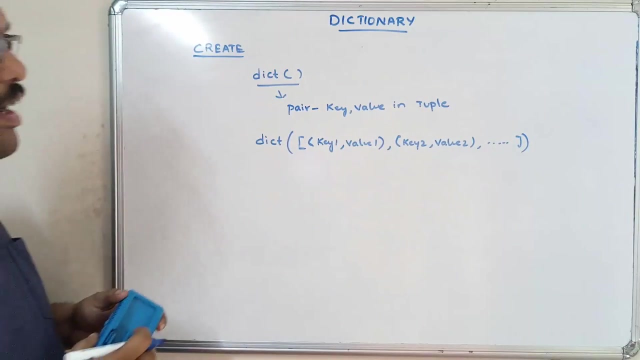 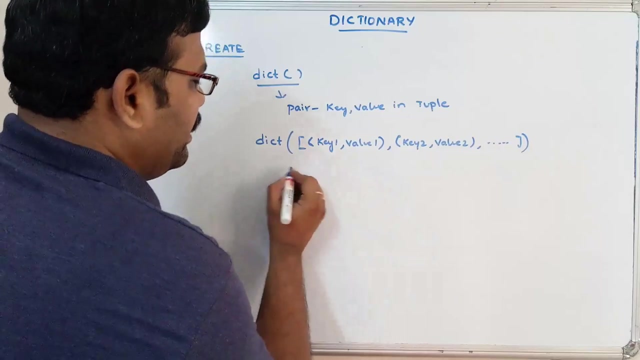 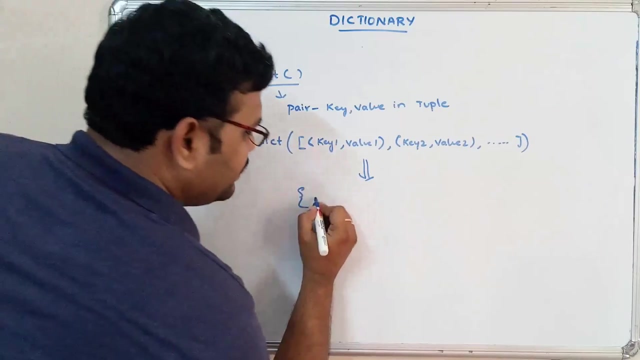 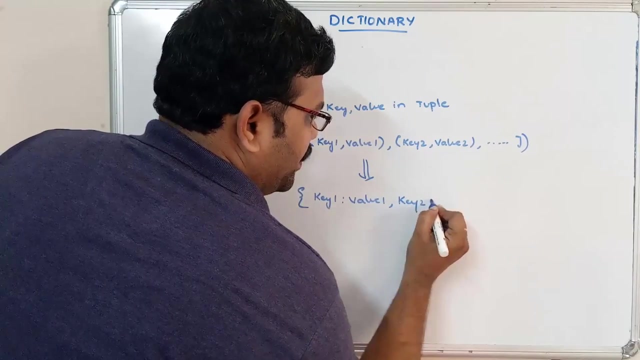 See, I will show you that DICT of key 1 comma value 1, key 2 comma, value 2, and so on. so in such a way we have to give the key value base. so this function will create a dictionary. this value will create a dictionary with the given syntax: so value 1 comma. key 2, value 2. 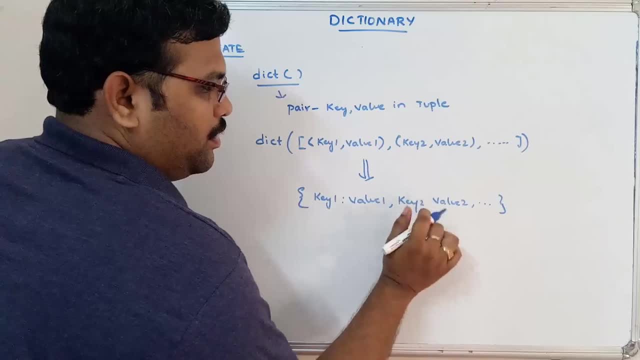 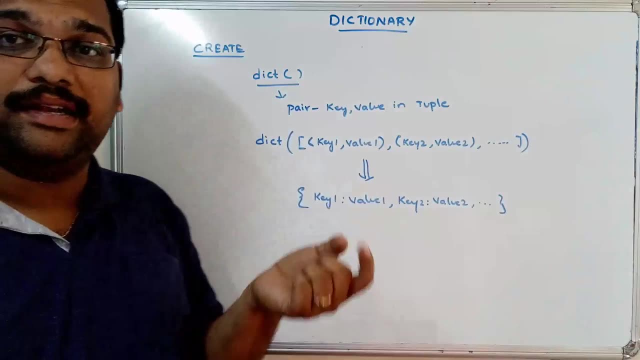 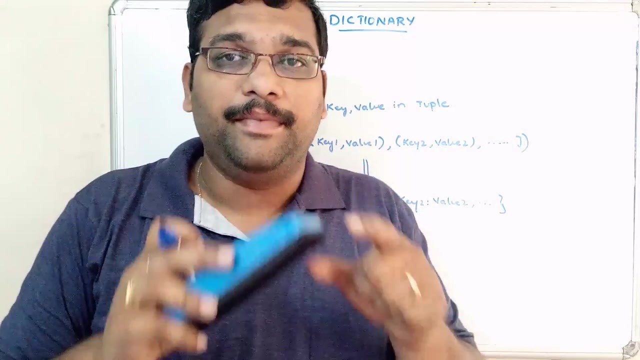 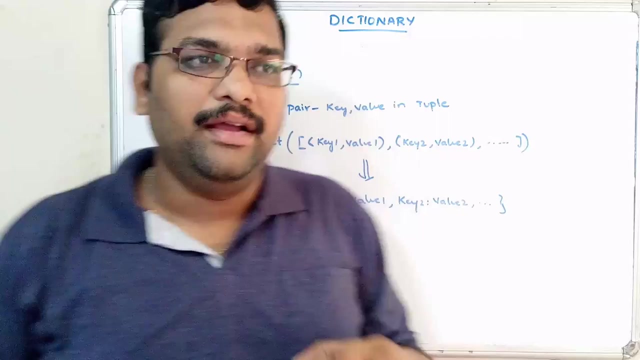 and so on. so it forms a. so directly we can. so we can create a dictionary, an empty dictionary. and we can create a dictionary by specifying the key value pairs in a curly braces in a single line, and we can create a dictionary with specifying the multiple elements and specifying each element in a single line, and also with the help of 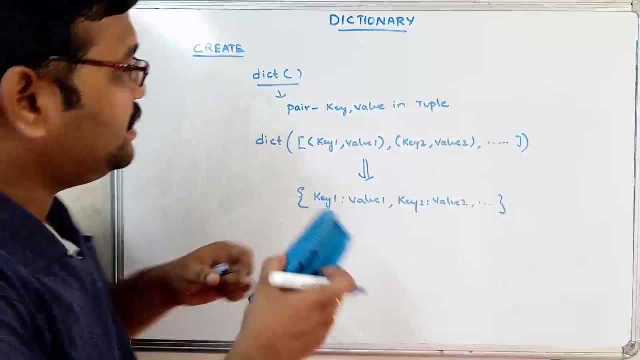 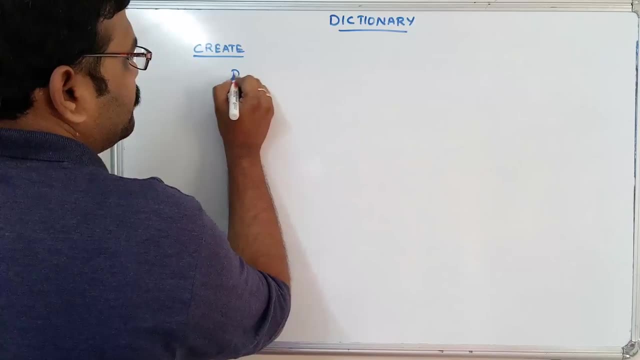 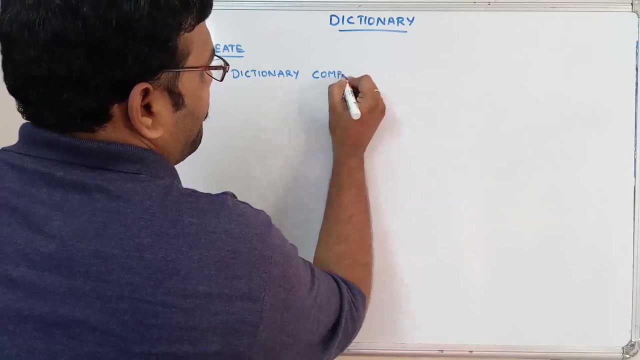 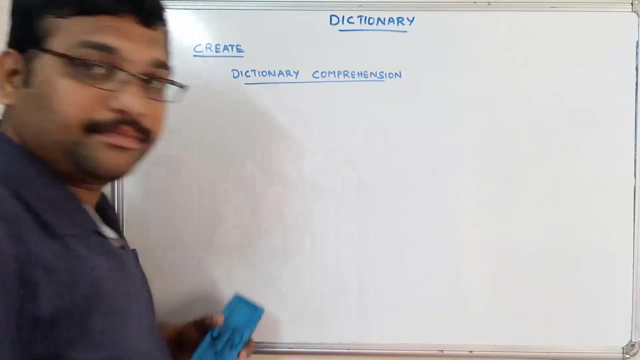 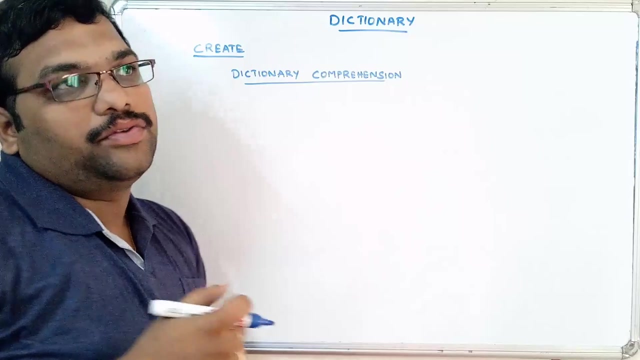 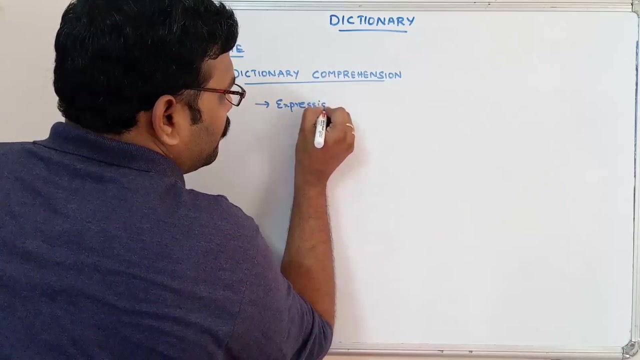 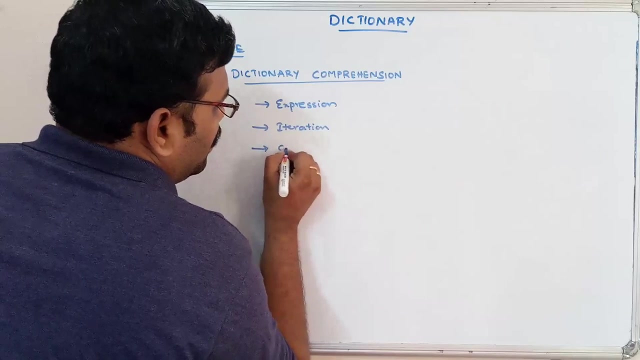 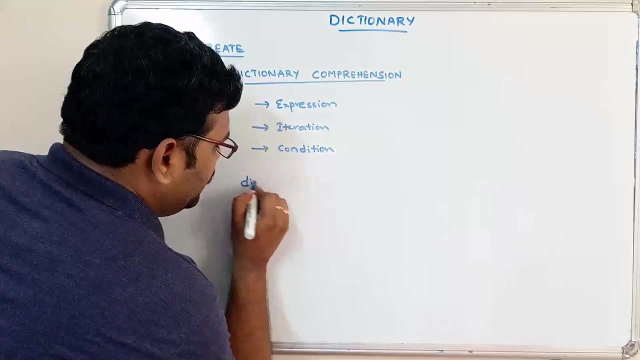 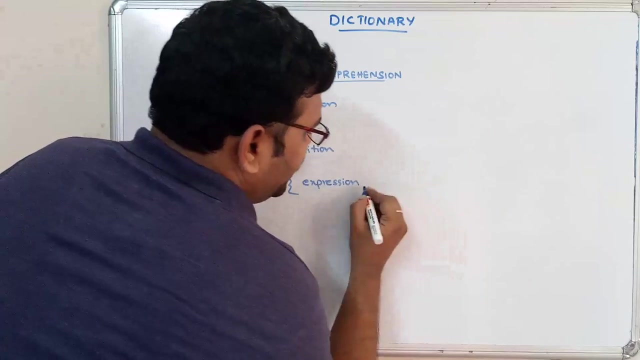 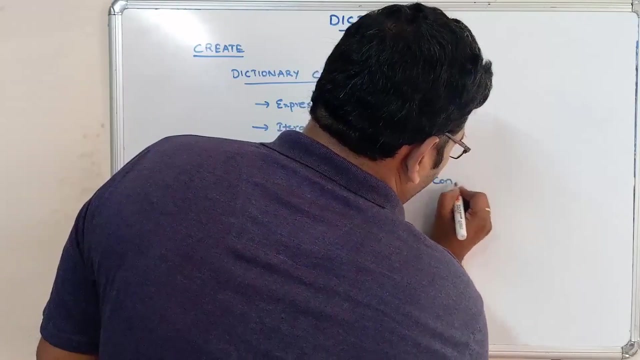 this dictionary function. and next we can also create a dictionary using comprehension. so we have seen this list: comprehension. so based upon the expression, the dictionary will be created. so we have to specify an expression iteration condition. so we have to follow the same order. so dictionary is equal to expression space, followed by iteration space, followed by condition. so 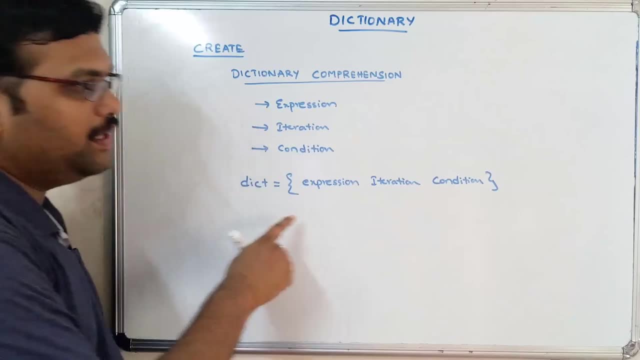 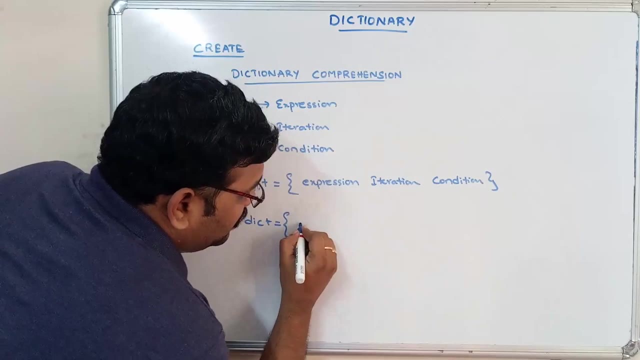 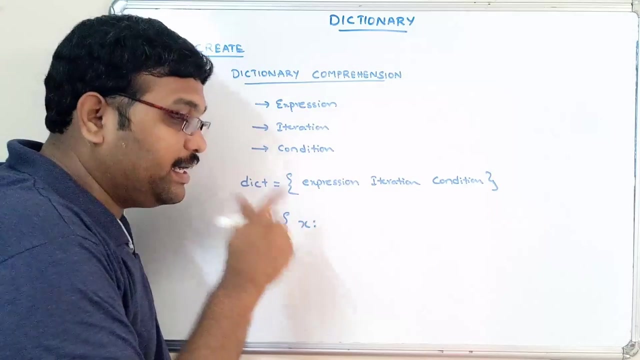 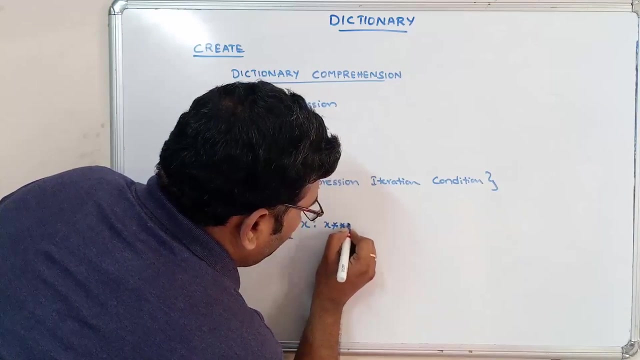 this is a syntax for creating the dictionary, with the use of list dictionary comprehension, for example. let me explain it with an example. some X pairs with: so this is a key value page, so we have to specify the key and a column and value. so X, star 2. 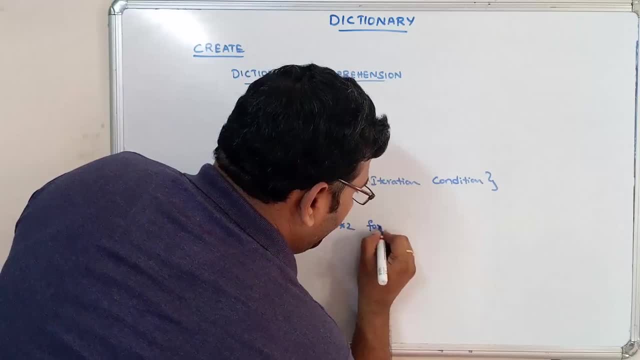 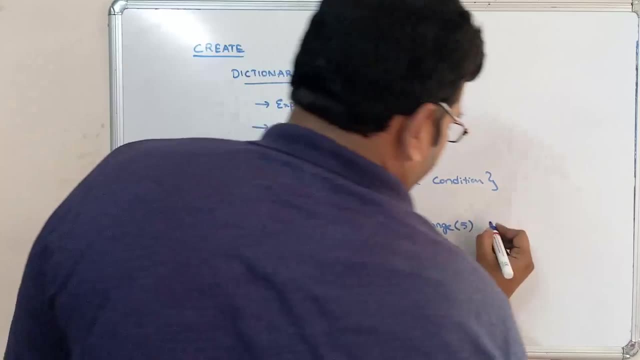 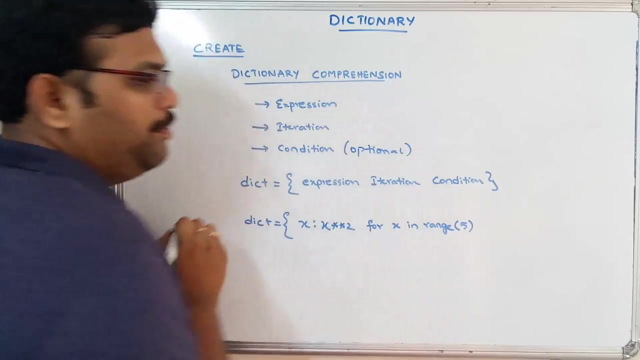 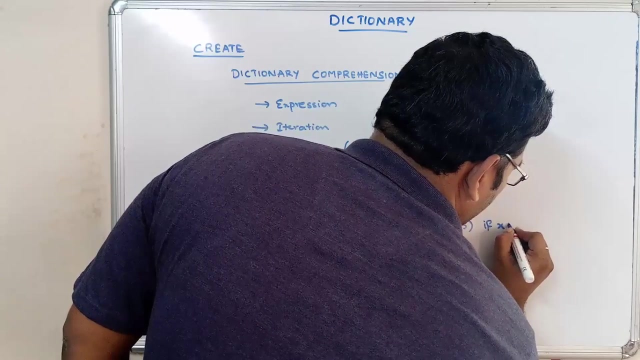 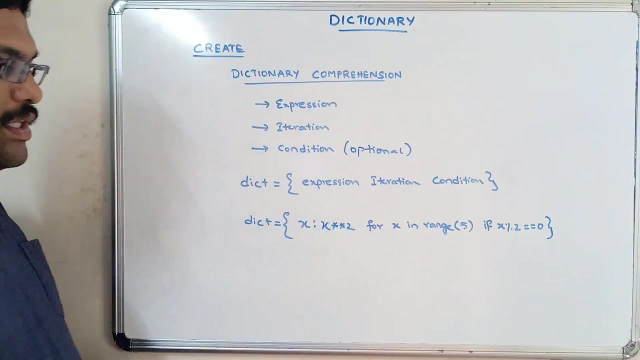 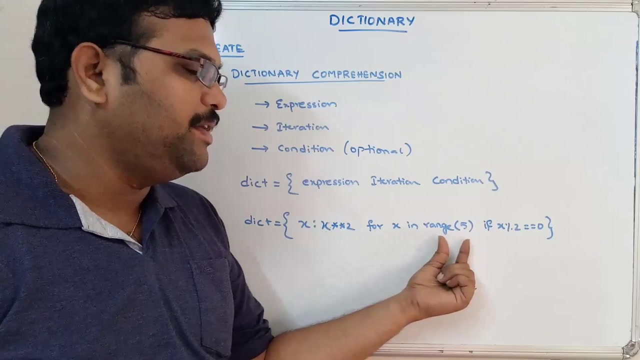 followed, but for X in range 5, and here this condition is optional. here the condition is an optional so we can use if développes we're going with, variable x is with zero. so we cannot use in normal terms sh followed based vaig by. So this implies we have to give the x pay for all the values of x in between 0 to 4, which are nothing but which mod 2 is not equal to 0. 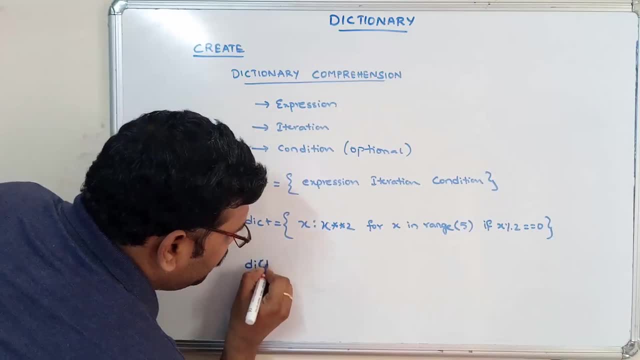 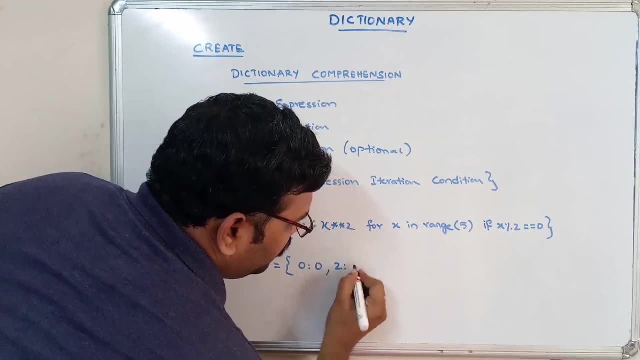 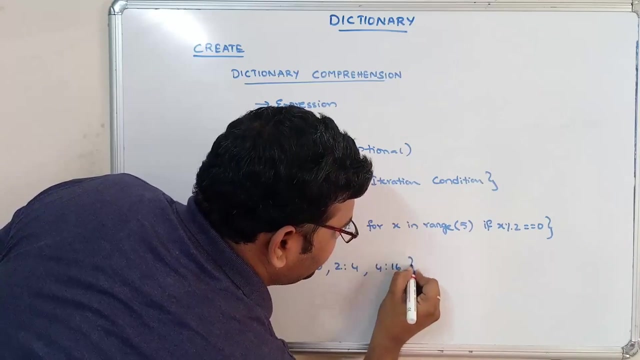 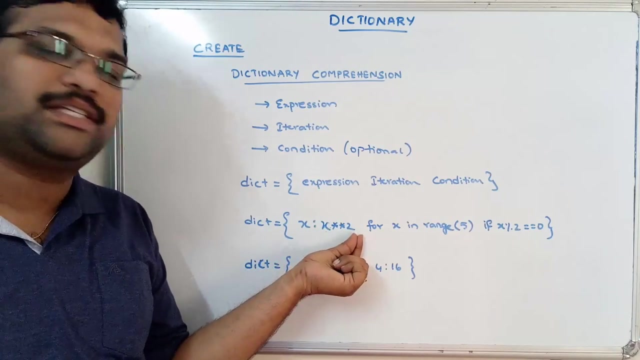 It means simply: it will fill 0, it forms a pay comma. 2, it forms a pay 4 and finally, 4, it forms a pay 16.. So it will give a result as this one. So x, colon, x, double star, 2, double star is nothing but our exponent operator, So it will be treated as x square. 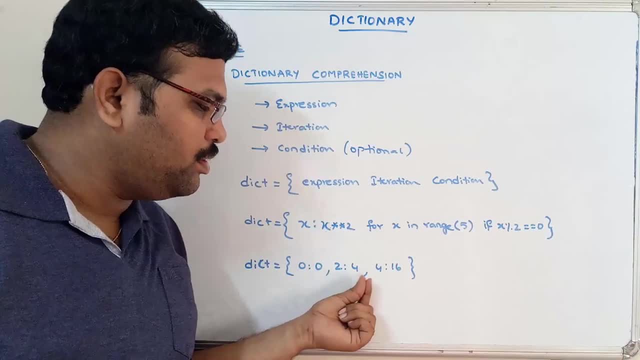 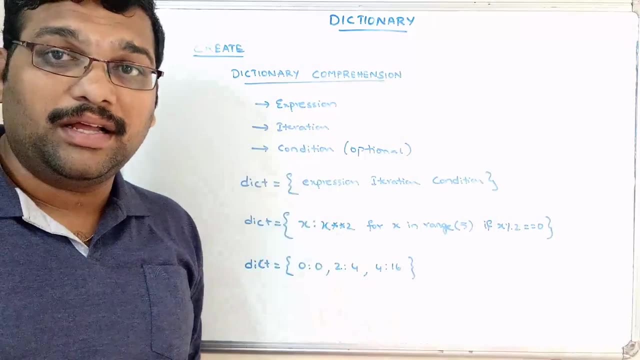 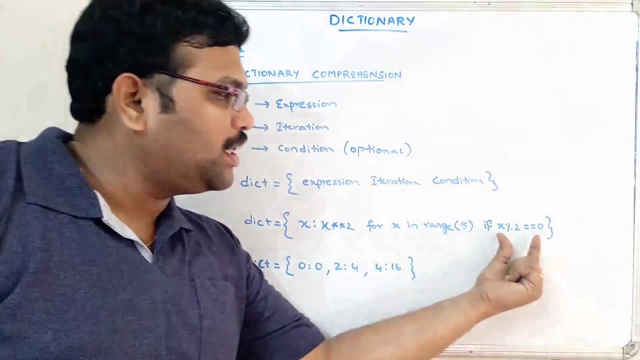 So 0, 0 square 0, 2, 2 square 4, 4, 4 square 16.. So because here we are giving the condition, x mod 2 is equal to is equal to 0. That means, whatever the elements which are modulated as 2 is equal to is equal to 0. So first the iterations will be executed and, based upon the condition, this will be inserted into the dictionary. 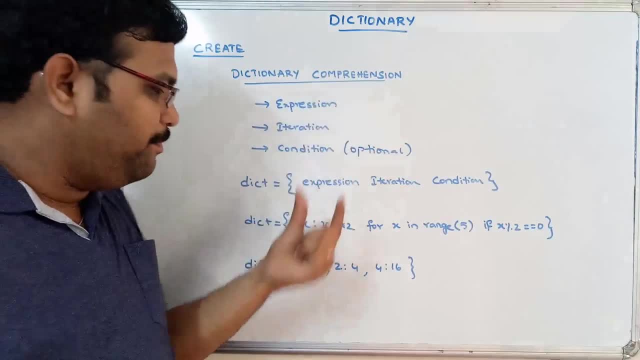 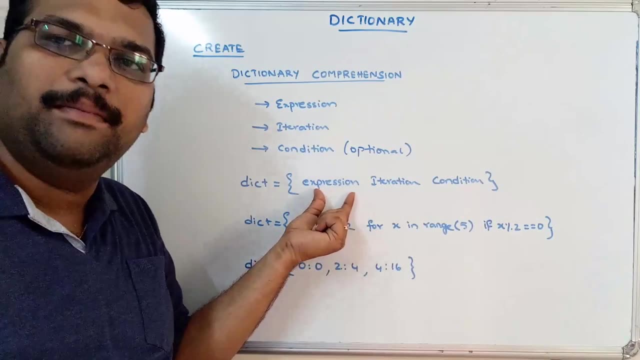 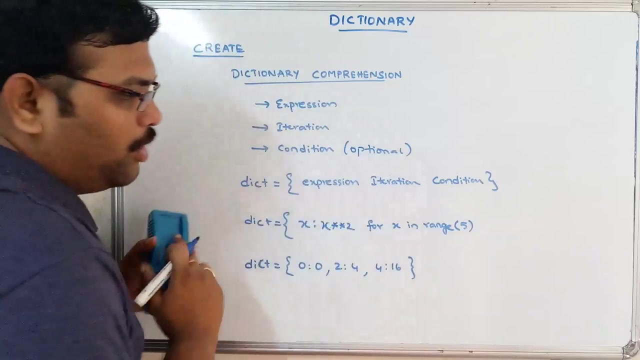 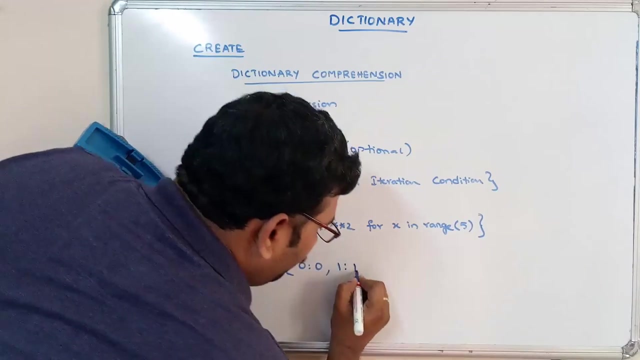 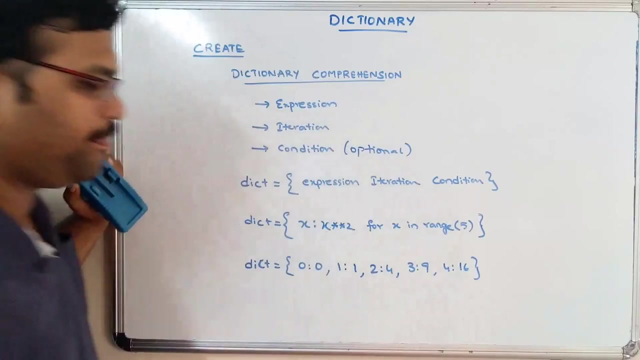 So this is called the dictionary comprehension. So while creating a dictionary, we can specify the condition and, based upon the condition, We can create an elements into the dictionary right. So if you are not specifying this condition, So here the condition is optional. If you are not specifying this one, So then the result will be 0, 0, 1, 1, 2, 4, 3, 9, 4, 16.. 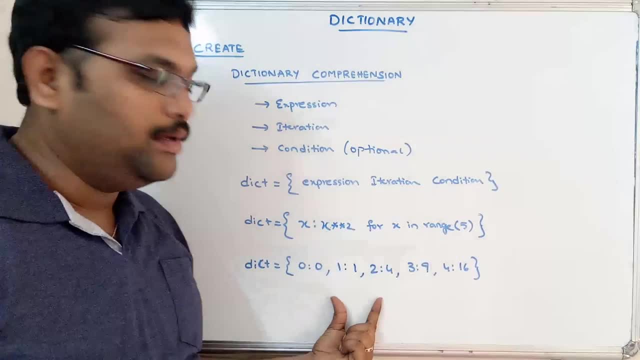 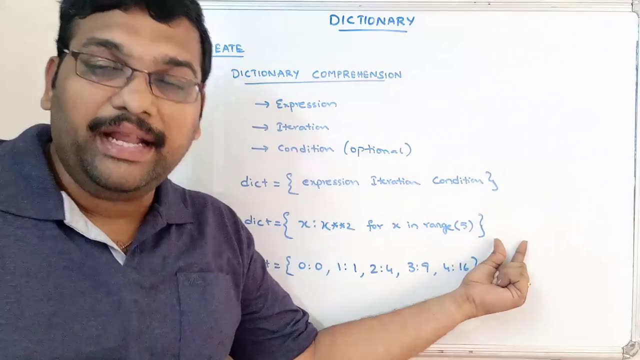 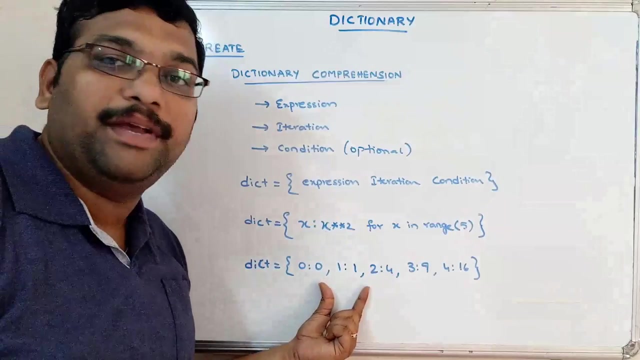 So this is the result for this comprehension, right? So first, always the iterative statements will be Executed. then, based upon the condition, if you are writing any condition, that condition will be verified and if the condition is true, then only the page will be formed and it will be created in the dictionary. 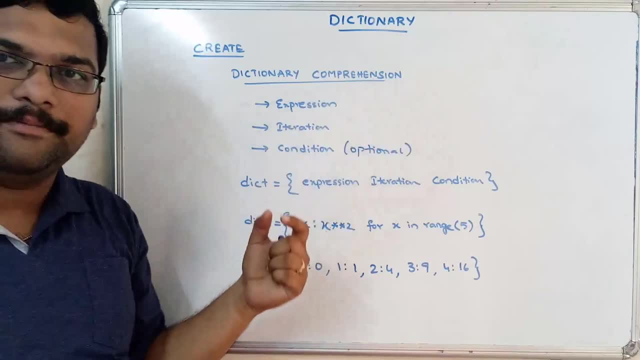 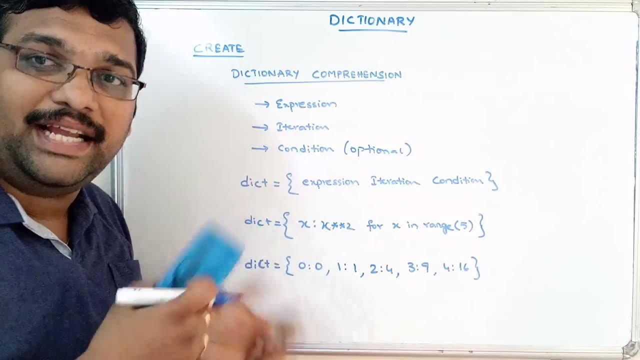 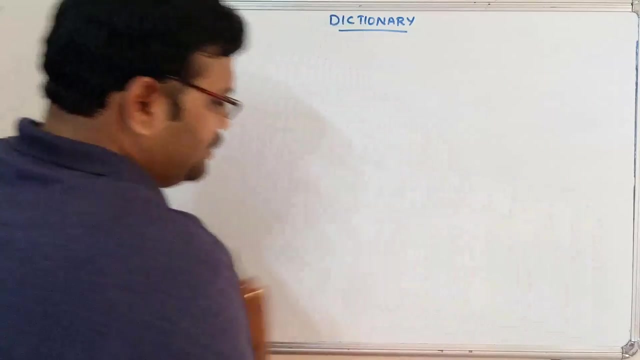 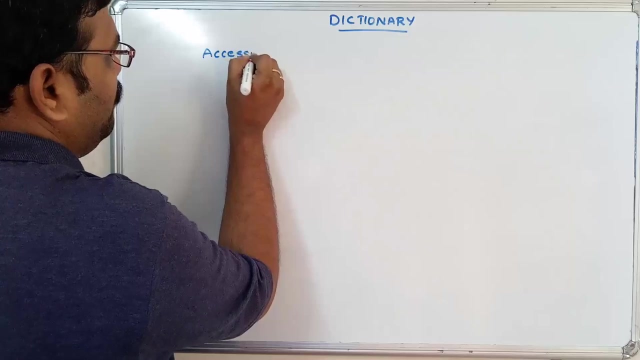 So this is how the dictionary comprehension will be working. So with the help of dictionary comprehension also, we can create a dictionary Right. So hope you understood this creation. how to create a dictionary. Now accessing How to access The elements or items of a dictionary. 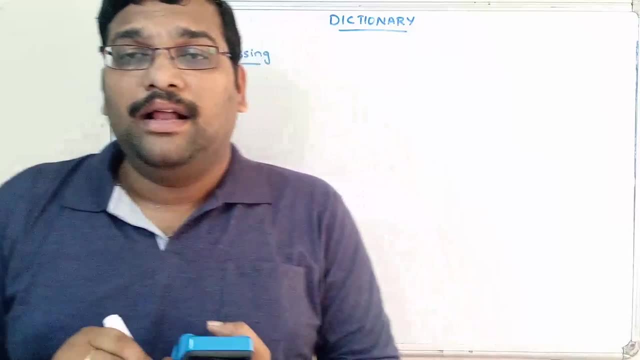 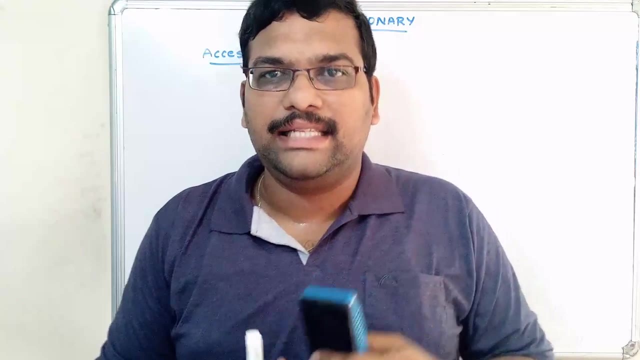 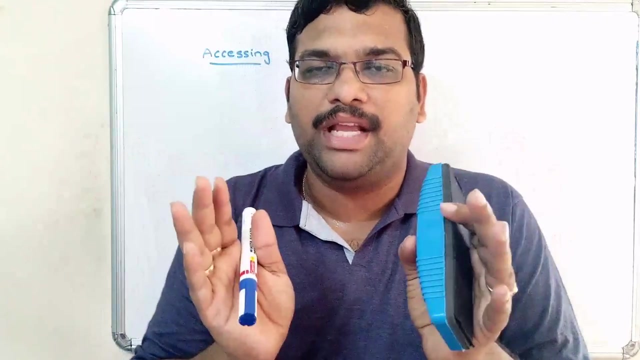 So, coming to this, previous sequences like list, tuples or set, So with the help of index values, will access the elements. So here we are having keys and values, a pair of elements we will be considering as a single item or single element. So here we are having keys and values, a pair of elements we will be considering as a single item or single element. 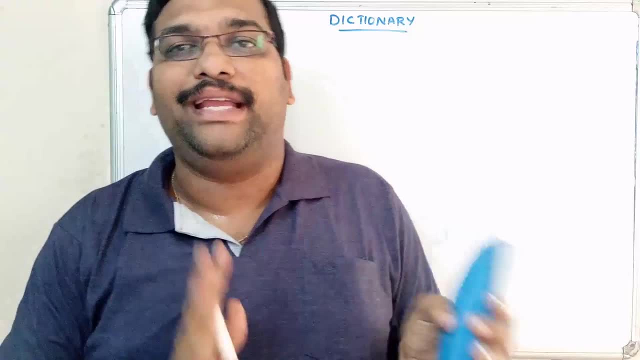 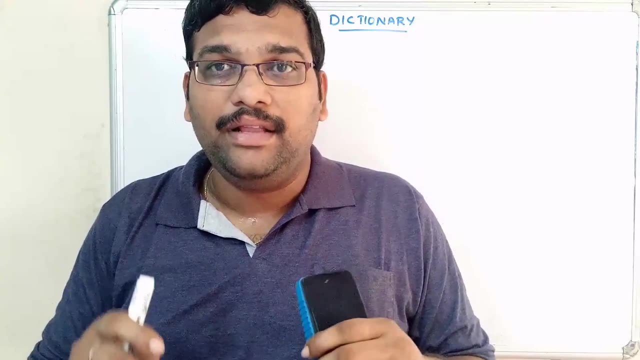 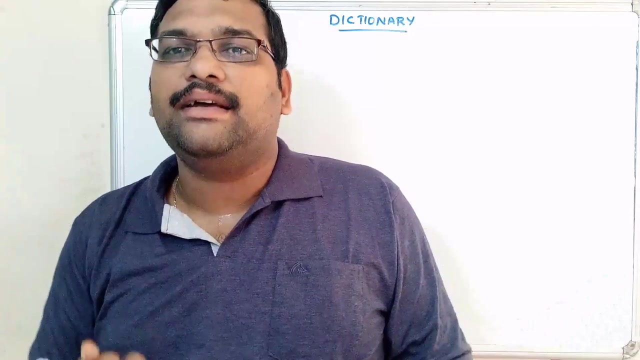 So we can access the values of a dictionary with the help of keys. So here there is no concept of index values. So here we are having the keys and values. So by using with the help of keys, we are going to access the corresponding values. 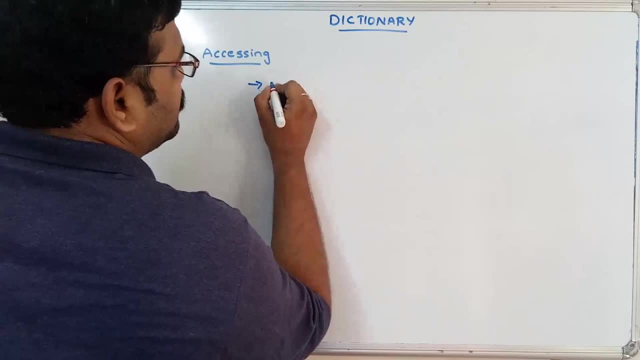 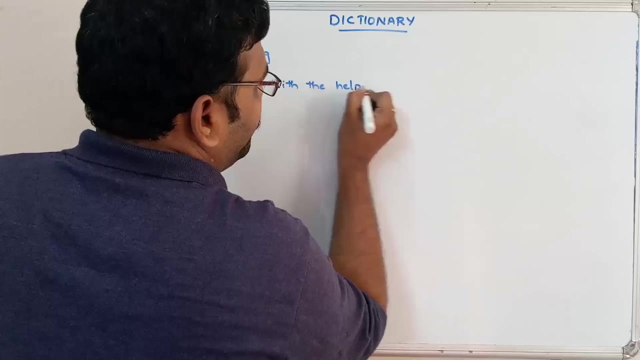 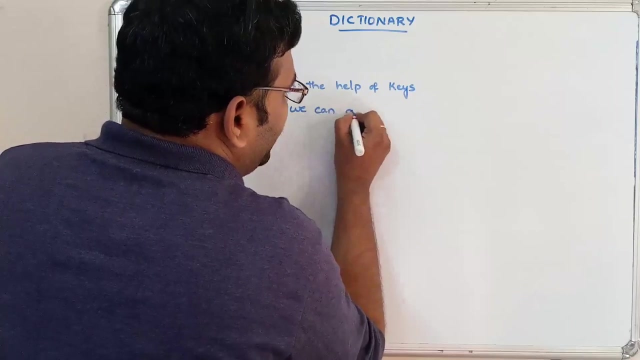 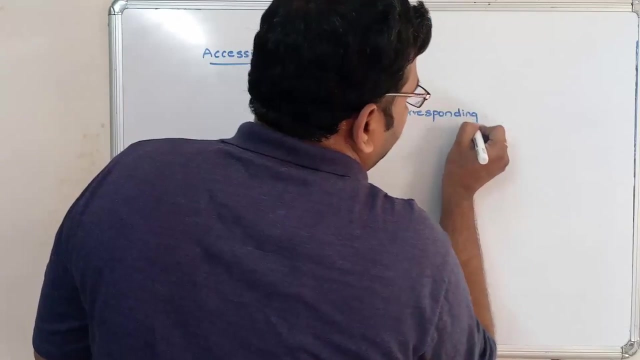 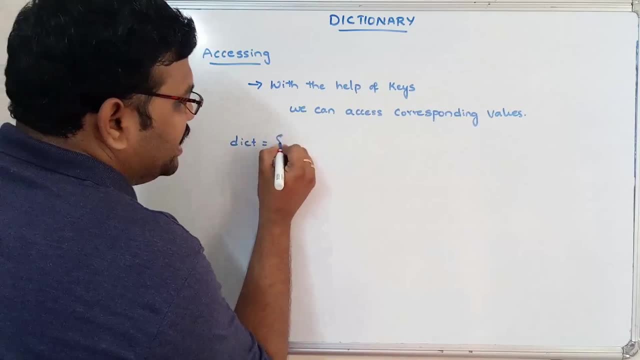 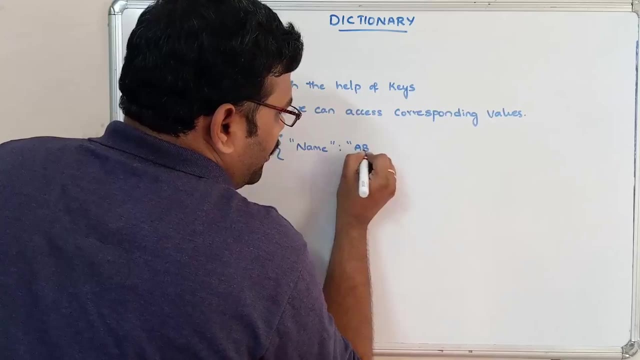 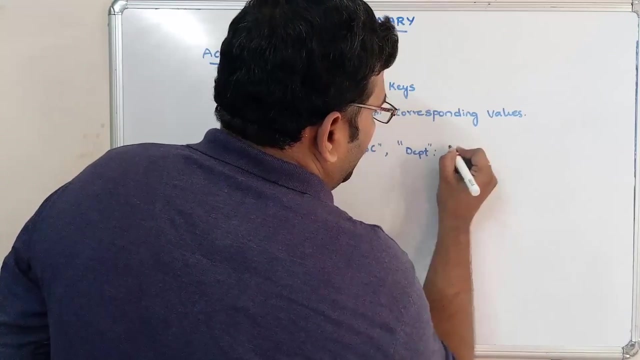 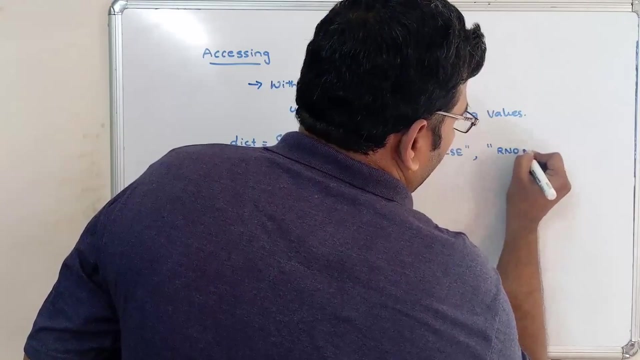 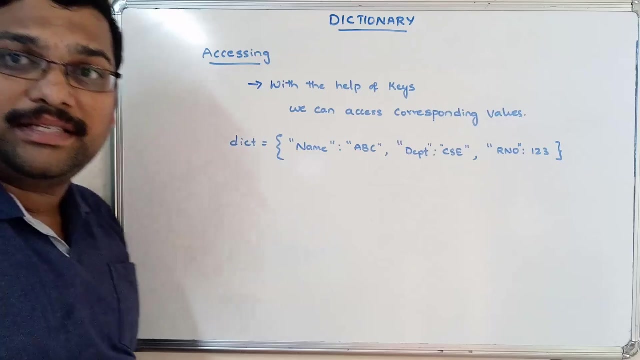 So, So, So We can access this. I will show you how this works, So I will try to show you So, So, So, So, So, So so there are three key value bits. okay, so this dictionary forms the three key. 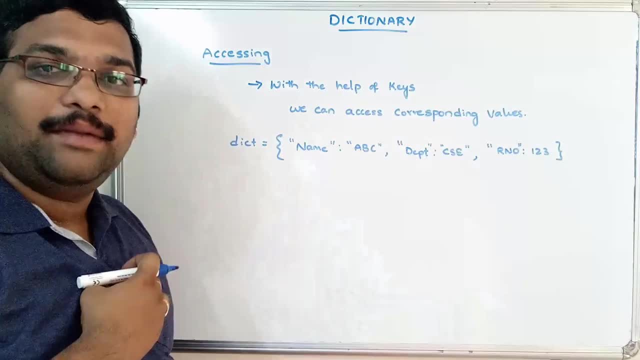 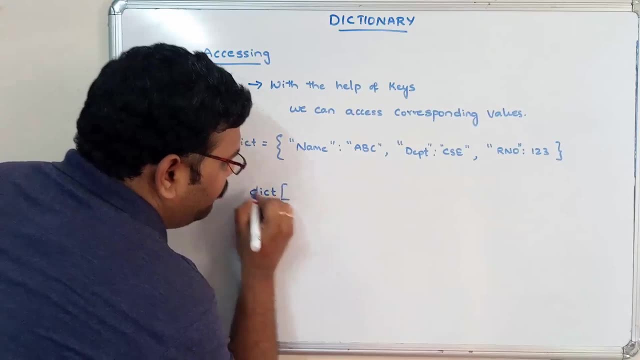 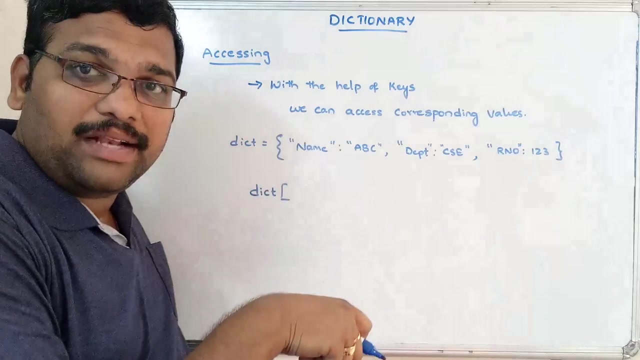 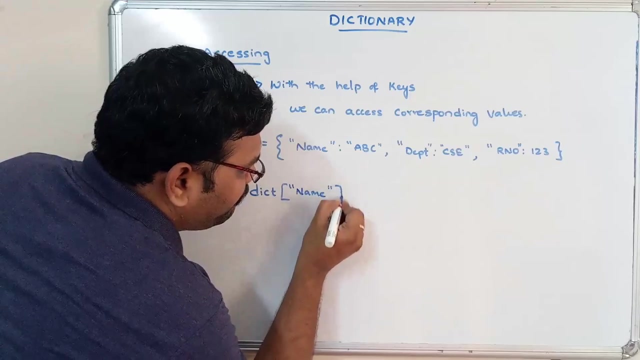 value bits. if you want to access these values, that can be done with the help of the corresponding keys. so DICT of. and here also we will use the square braces for accessing the element. so in the square braces, instead of writing this index values, here we will write the keys. so dictionary of name. similarly DICT of. 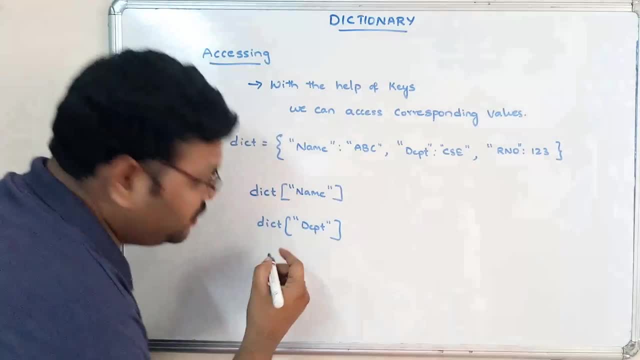 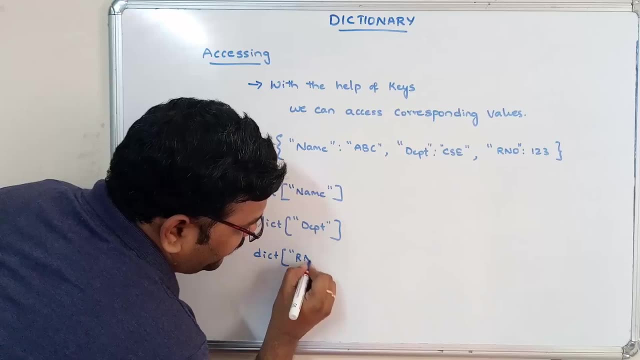 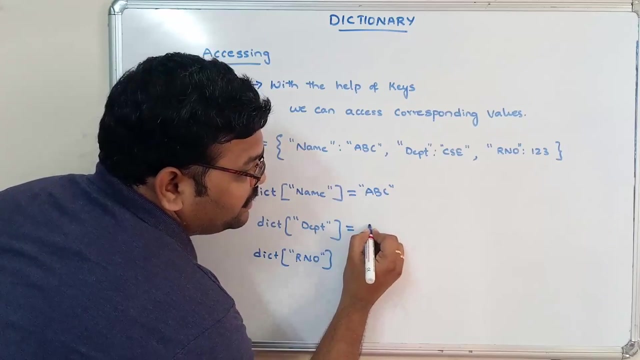 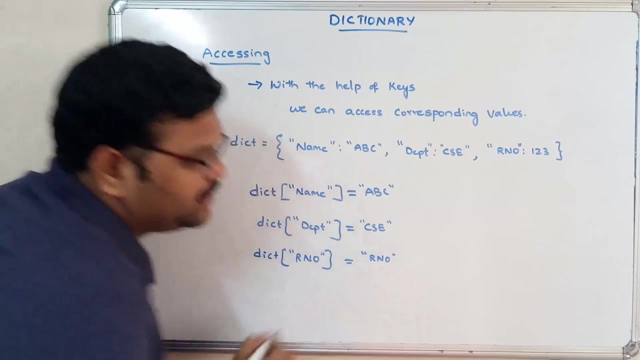 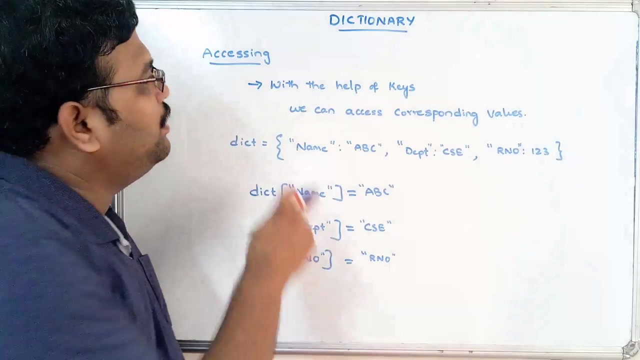 DEPT. so this is a string. so we have to enclose in quotations dictionary of R number. so this will return everything as a result, and this will design return C SC as a result, and this will return R number as a result. okay, so this is how we can access the elements of a dictionary. so 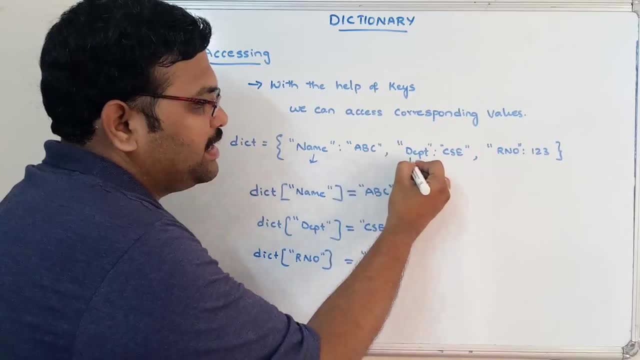 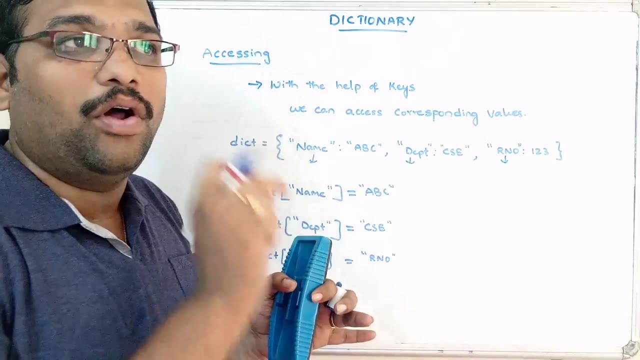 with the help of оно, the keys. so all these are the keys. okay, so all these are the keys. that means the left hand side, which we are writing to the column, those will be considered as a keys, and right hand side are the corresponding values. so, with the help of